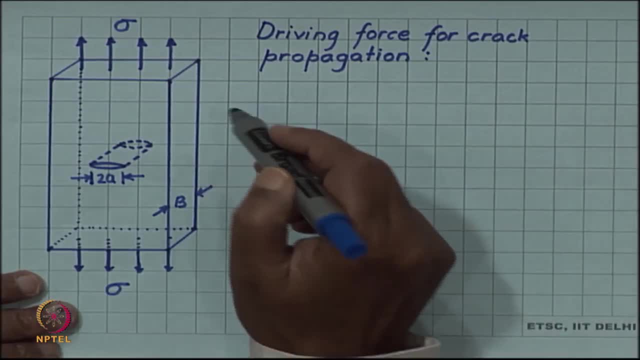 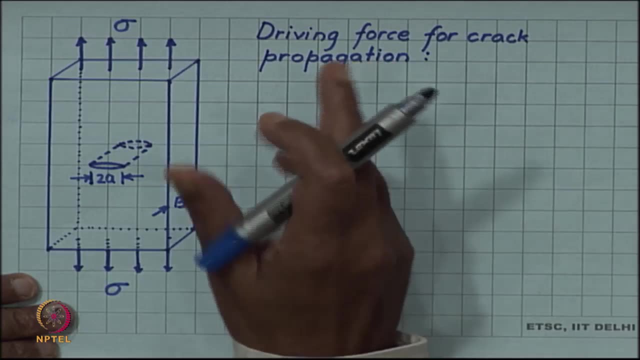 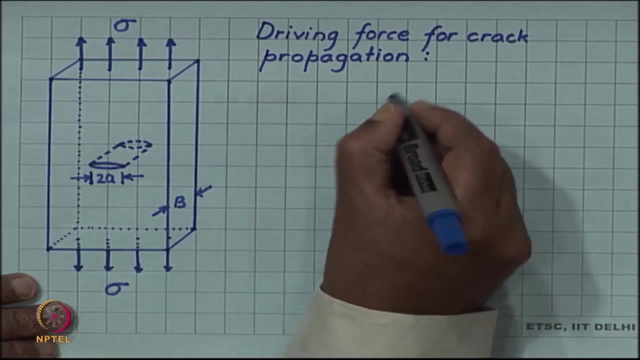 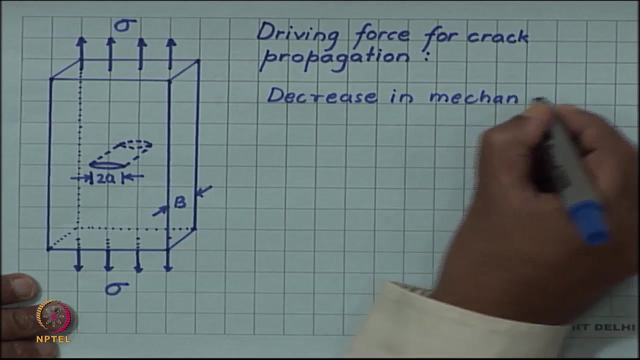 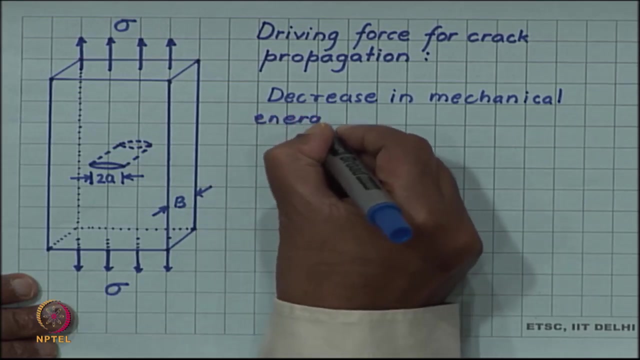 propagate What energy is decreasing? So Griffith could see by his analysis that the energy which is decreasing in case of crack propagation is the mechanical energy of the crack. The system driving force for crack propagation is decrease in mechanical energy. Mechanical energy has two. 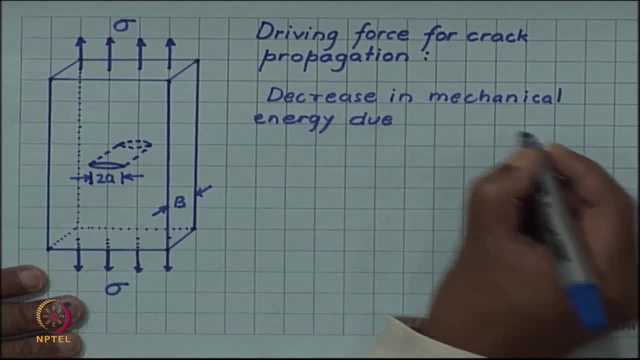 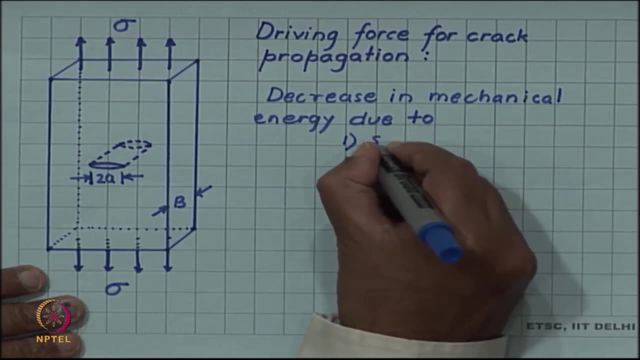 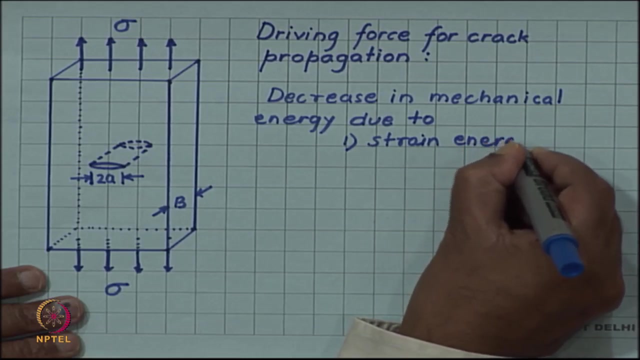 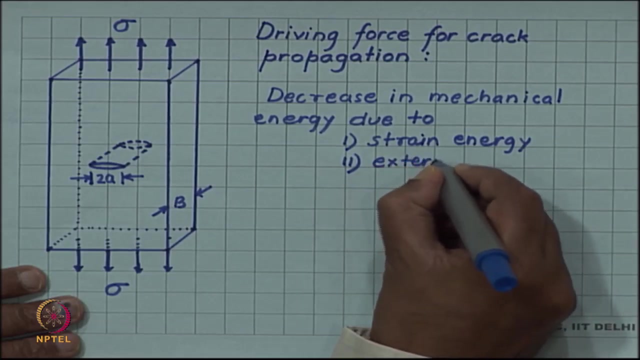 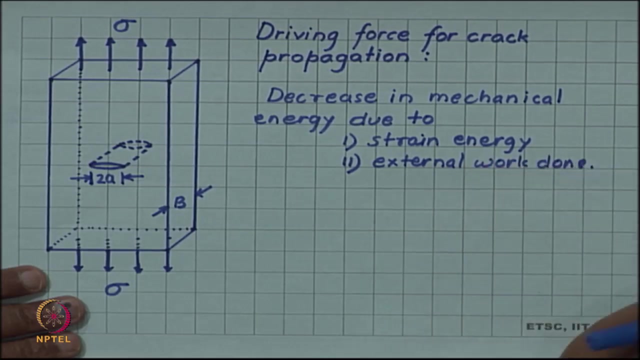 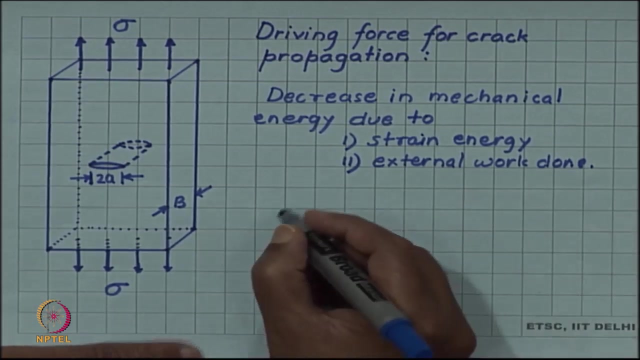 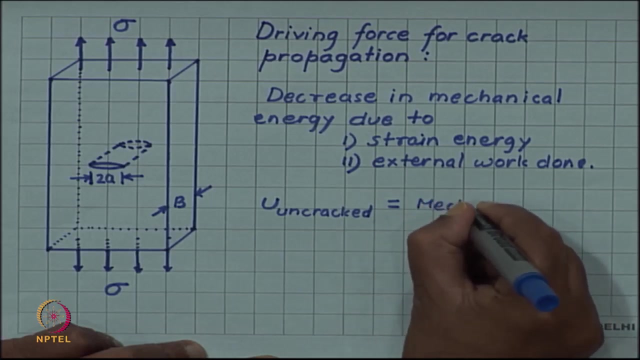 two components. we will not go into the details of this, So we just write: decrease in mechanical energy due to strain energy, elastic strain energy and external work done. So since this mechanical energy reduces or decreases, let us write that U uncracked is. 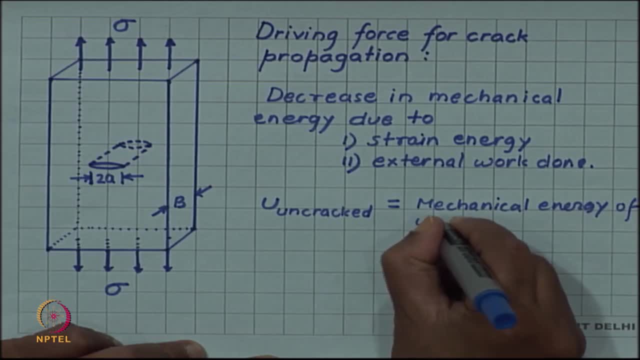 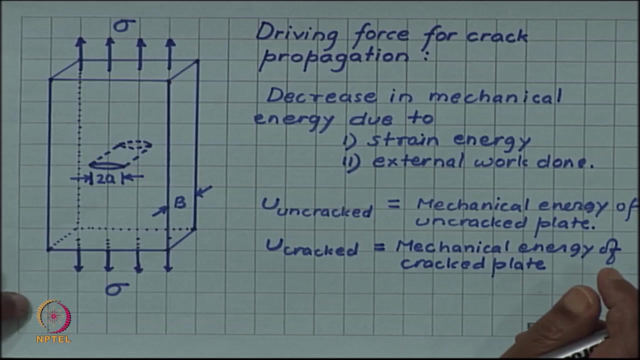 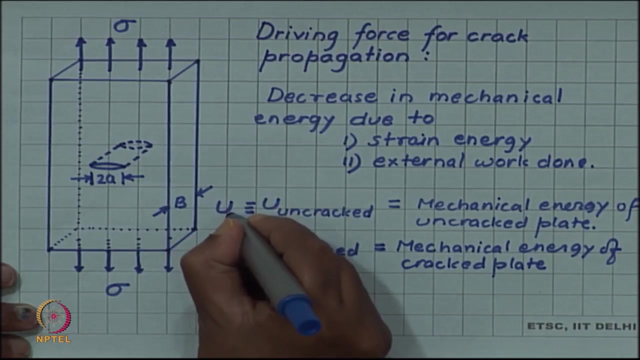 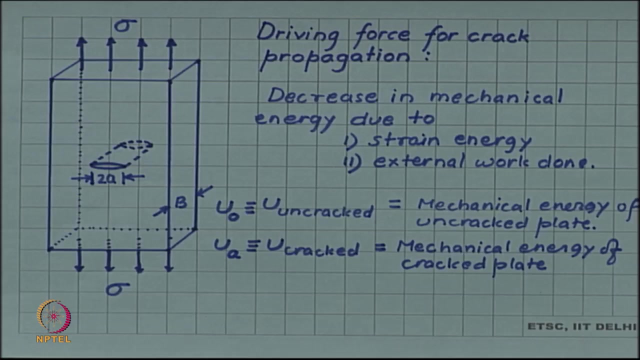 mechanical energy of uncracked plate and U cracked mechanical energy will increase or decrease. So notice this coобы plate. maybe I use a simpler symbol. So for uncracked let me write u o, that is crack of 0 length is there. and in crack I write u a, that is crack of length 2 a is there. 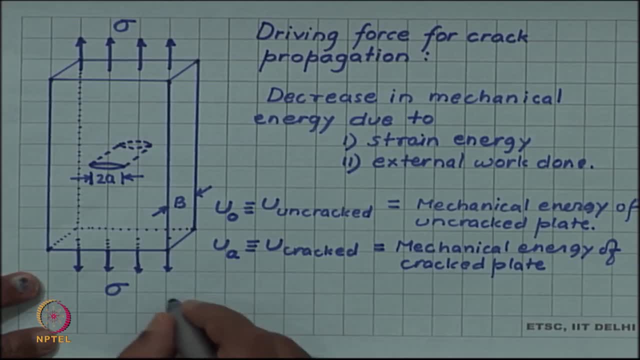 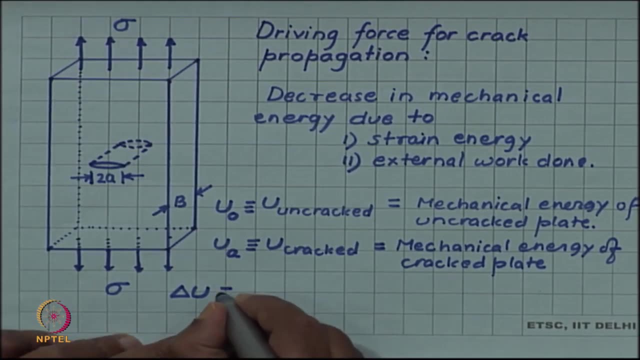 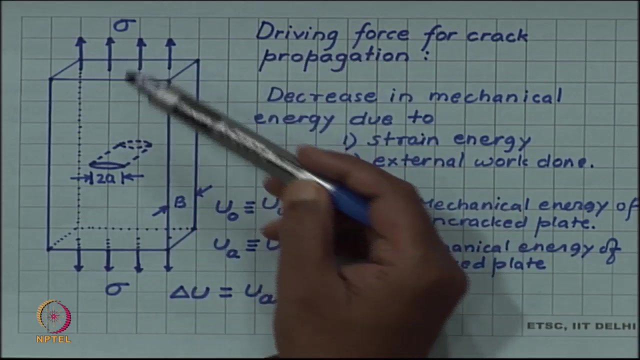 Now that, So the change in mechanical energy, the change in mechanical energy due to the introduction of the crack, can be written as delta u, which is u with crack, delta u with minus u without crack, and this can be calculated in terms of the stresses, the crack size. 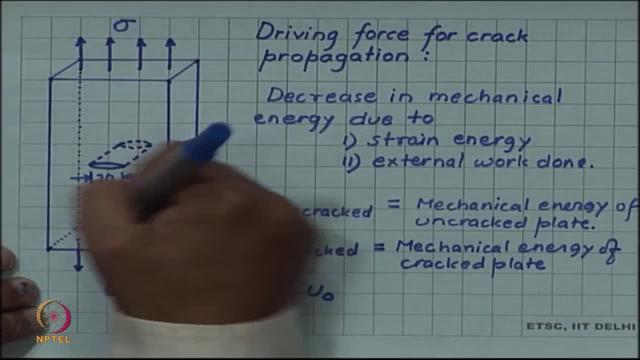 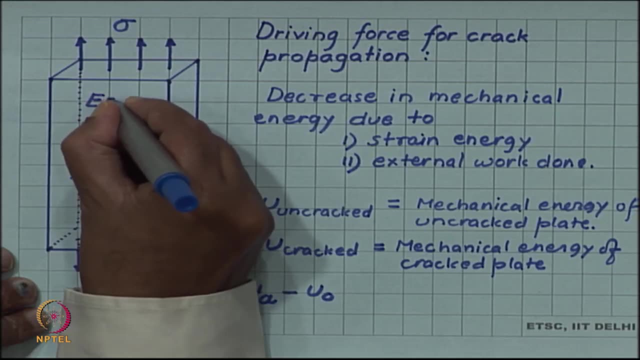 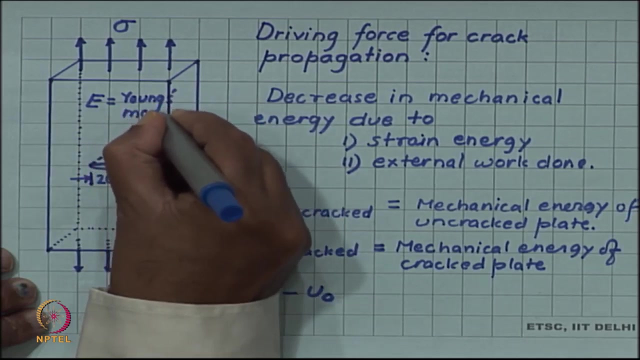 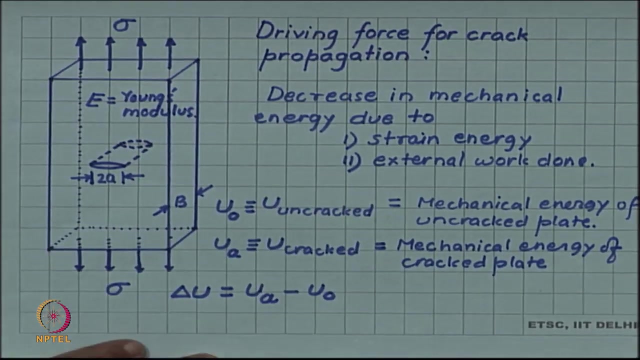 the plate: thickness and the elastic property of the material, which, in this case, is the Young's modulus. So let me write E as the Young's modulus of the plate. E is the Young's modulus. So, in terms of these parameter, if I, if it is calculated, 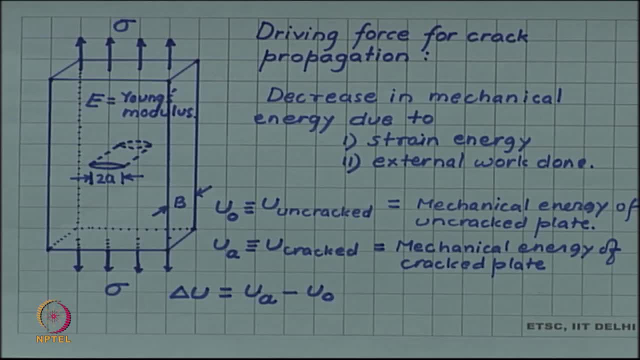 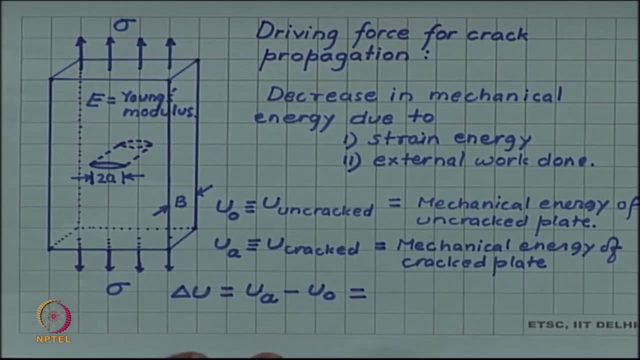 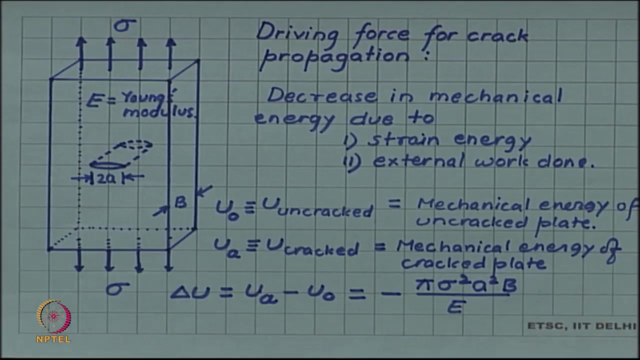 now the calculation is much more involved. it is a problem in solid mechanics or continuum mechanics. we will not get into that. We will simply take the result from the calculation of Griffith. and that is minus pi. So this is the difference in the mechanical energy. negative sign shows that the mechanical 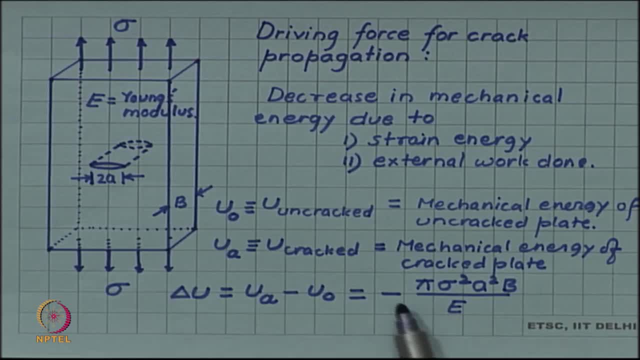 energy is decreasing and mechanical energy is decreasing by this much amount, that is, it is pi times square of stress, times square of the crack, Square of the crack length, or half crack length times the thickness divided by the Young's modulus. So higher is the applied stress, more will be the decrease in elastic. 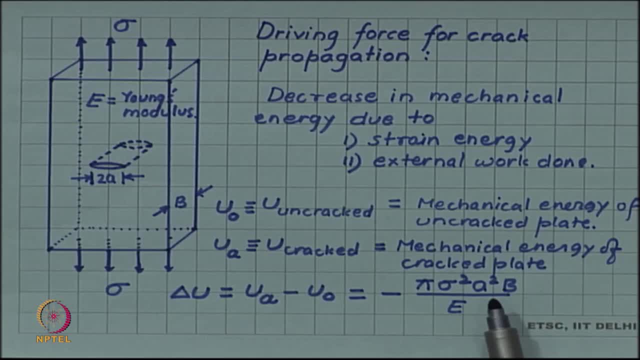 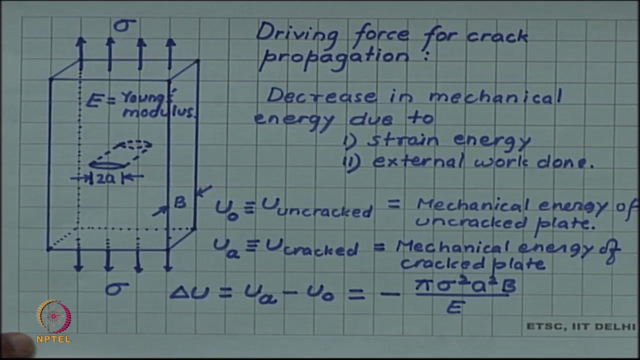 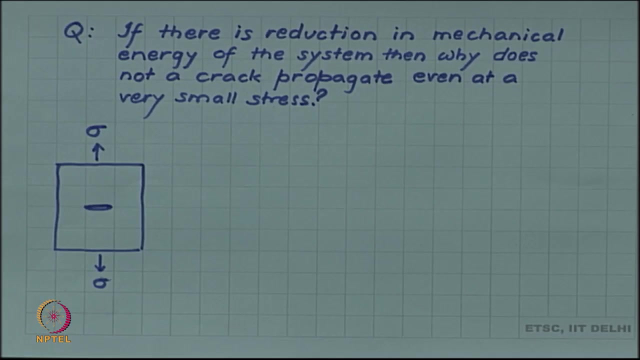 energy. higher is the crack length, more will be the decrease in elastic energy. higher thickness will also lead to greater decrease in elastic energy, But higher modulus will leads to lower decrease in elastic energy. So this is the driving force. this is the driving force for crack propagation reduction. 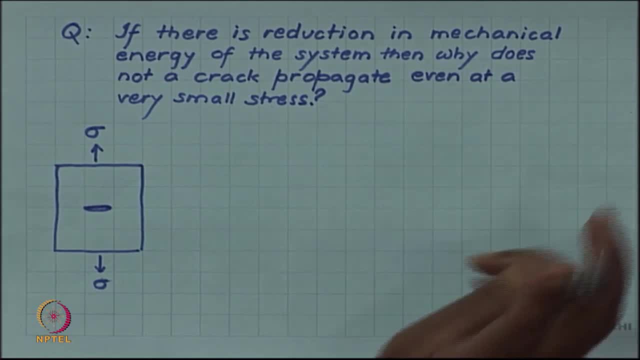 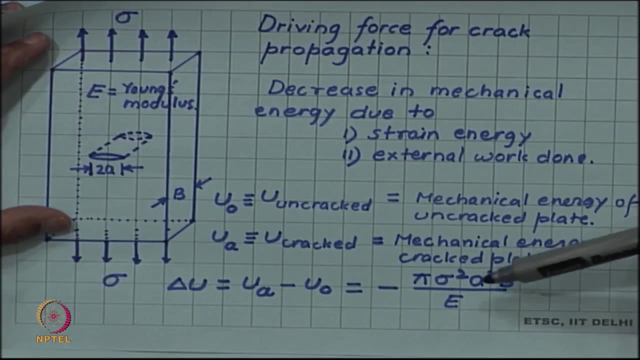 in mechanical energy. But then the question comes if there is a reduction in mechanical energy, and you can see from this formula that for a given crack size, whatever is the strength, whatever is the strength of the crack, whatever is the strength of the crack, whatever is. 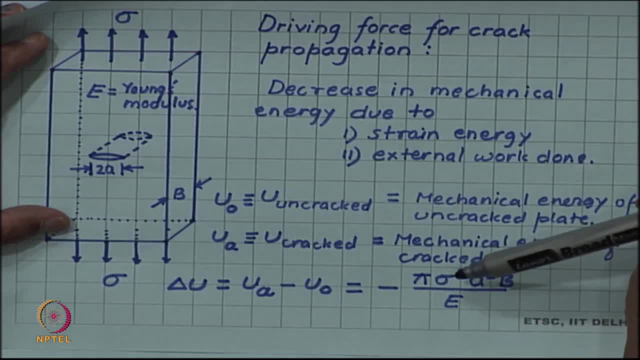 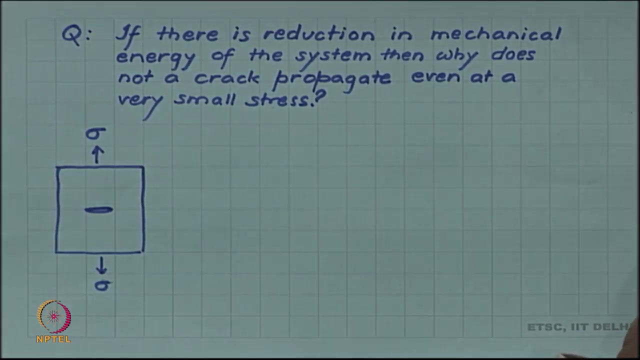 the stress, however small the stress is, there will always be a decrease in energy. So whatever be the crack size and however small stress I apply on it, there will be a decrease in mechanical energy if the crack propagates. But we have just seen in the paper experiment. 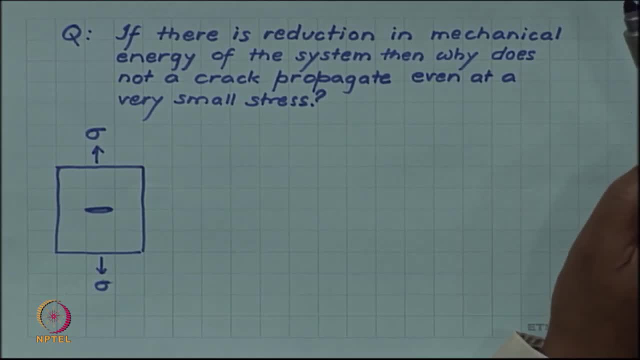 and we know from our experience that even if crack is there, the crack will not propagate unless and until the applied stress is certain critical value. Very small stress, very feeble stress, will not lead to crack propagation. So if there is a reduction in mechanical energy of the system, then why does not a crack propagate? 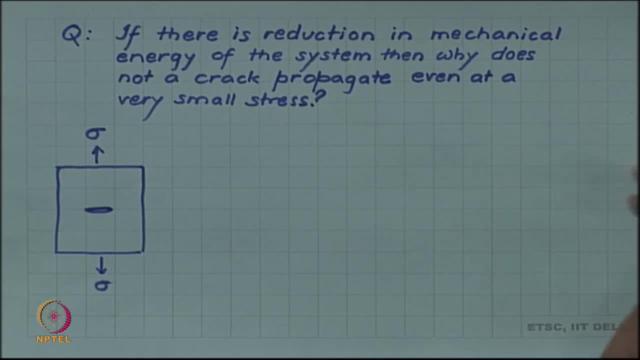 even at very small stress. So this was an important question. this was an important question which Griffith asked and he came to a very, very interesting answer. What he realized? That mechanical energy is only one aspect of the energy of the system. The other aspect 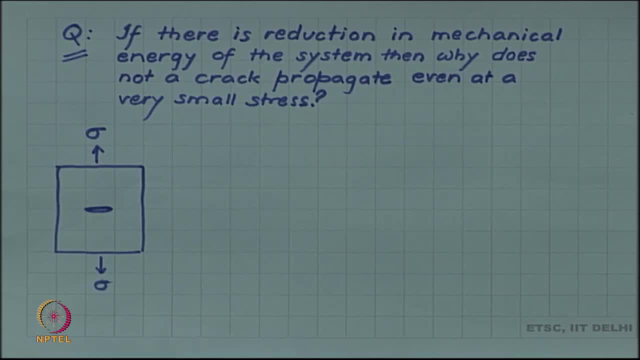 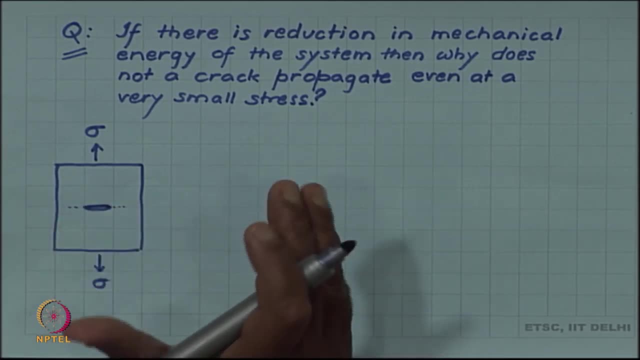 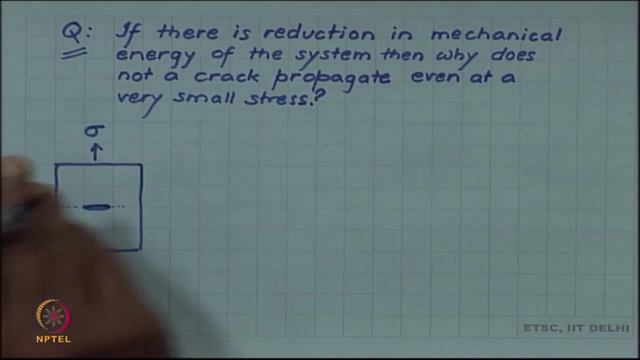 of the energy of the system is its surface energy. As the crack will propagate, or as you introduce the crack, you also introduce two free surfaces, two surfaces of the crack. So let us write that with the introduction of crack, 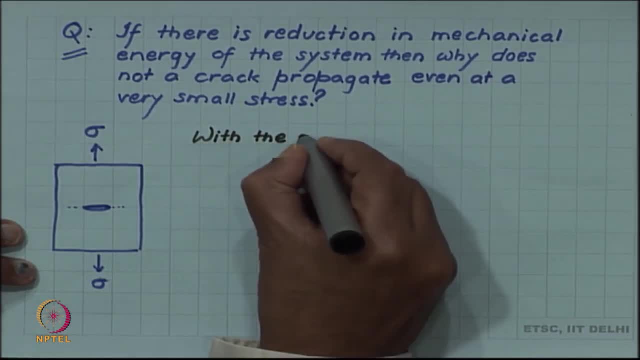 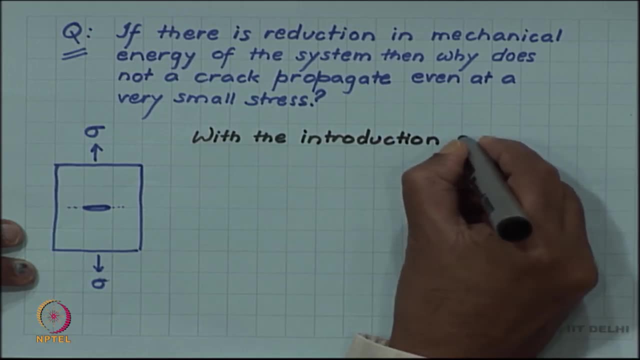 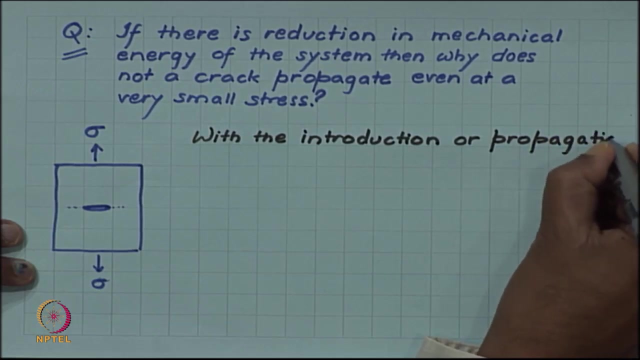 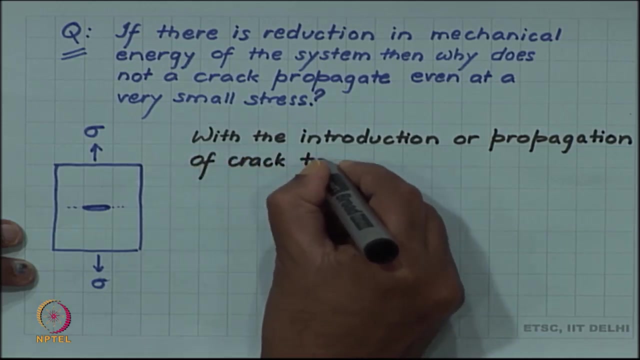 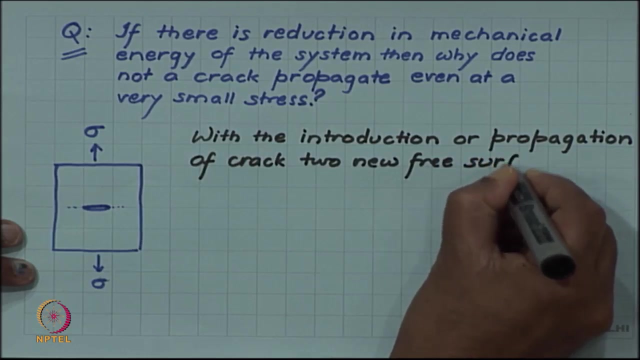 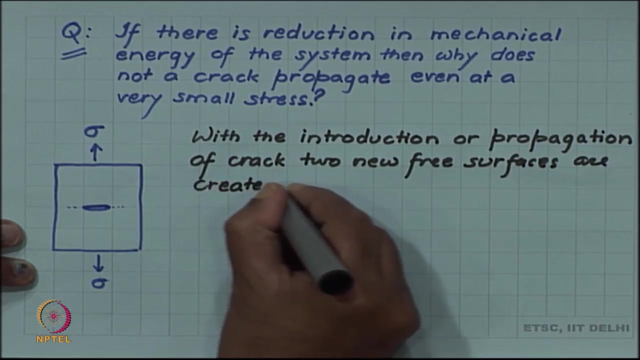 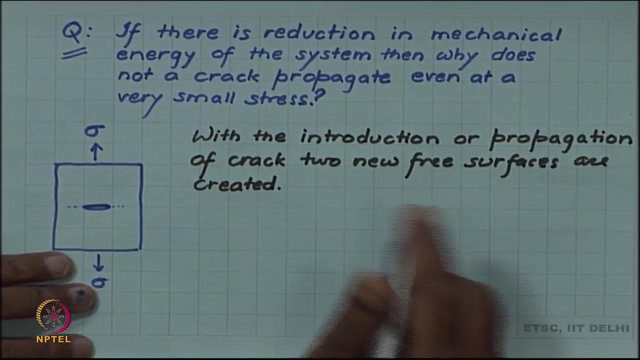 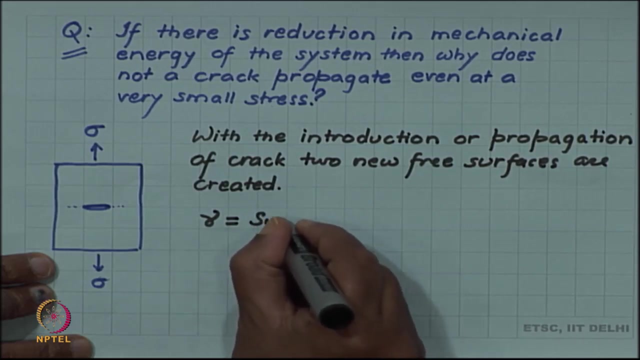 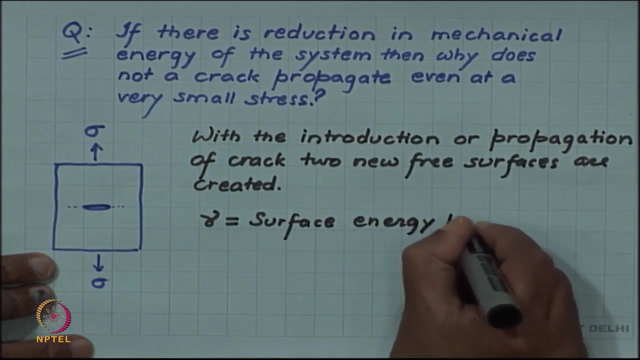 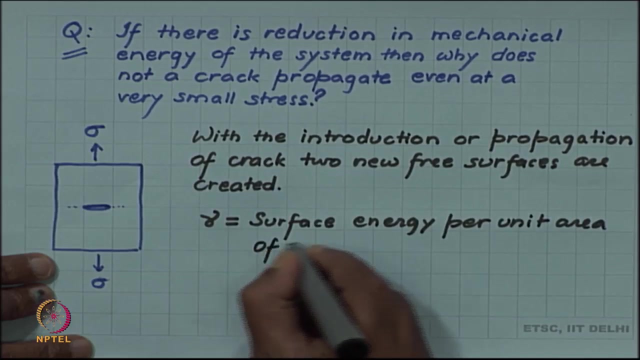 with the introduction or propagation of crack to new free surfaces are created, And we know that every free surface is associated with a positive surface energy per unit area. So let gamma be the surface energy per unit area. So this is a very, very interesting concept. this is a novel concept. this was novel concept. 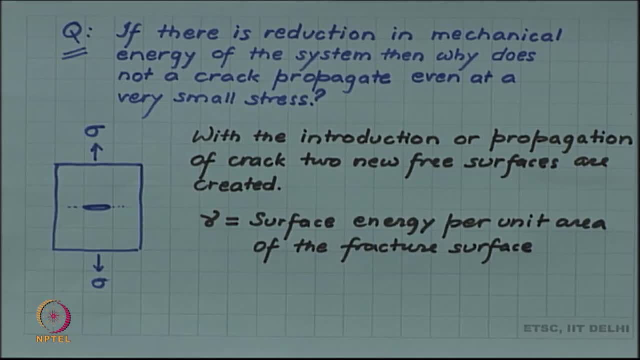 at the time of Griffith, before Griffith, no one had realized about this and nobody had introduced this into the analysis of fracture. So it is a central importance to Griffith So in his analysis that he introduced the concept of surface energy, of the fractured. 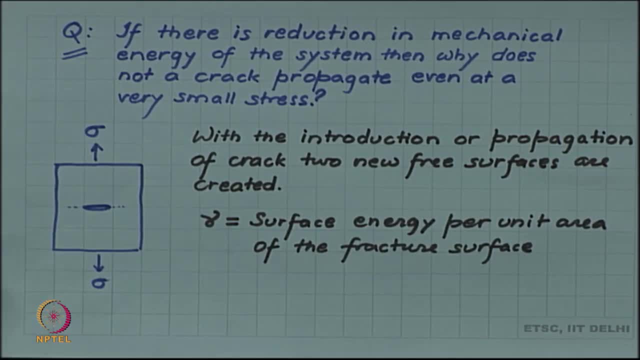 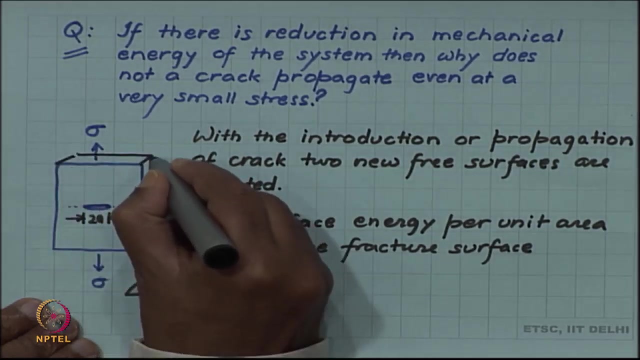 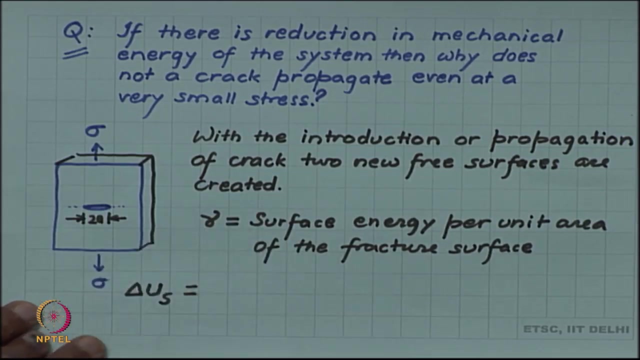 surface into the analysis of crack propagation. So with this we can now write that there is another energy change component. let us write that delta U surface. So if we introduce a crack of length 2 a in a plate of thickness b, how much new surface? 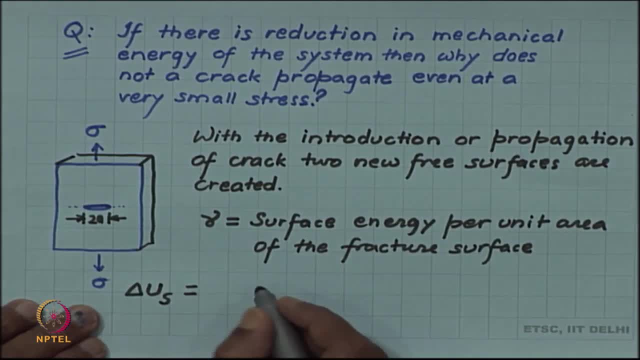 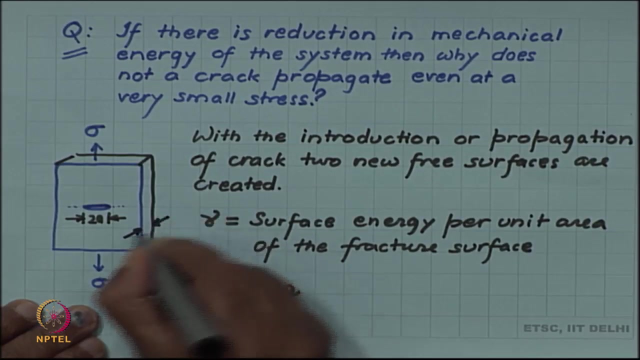 say energy we have introduced. So we can see that we have created two surfaces. So let me write a factor 2.. So, and each surface is of length, 2 a and width b, width equal to the thickness of the plate. 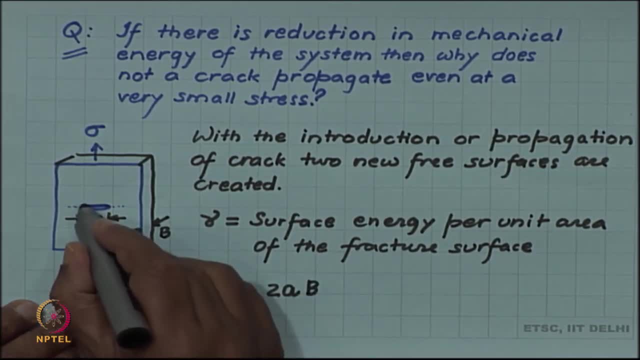 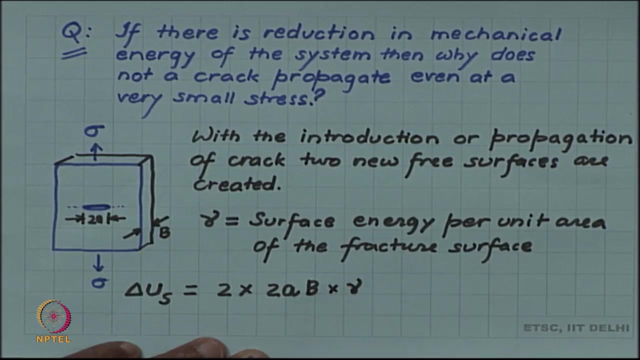 So 2 a b is the surface area of the upper surface, 2 a b is the surface area of the lower surface. So 2 times 2 a b is the total surface area created and since gamma is surface energy per unit area, 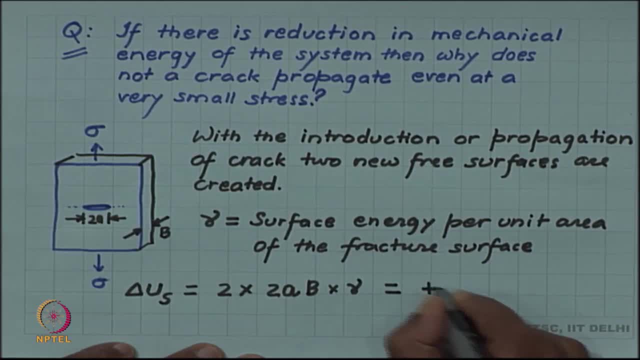 So we see that there is an increase in the energy equal to 4 a b gamma due to the crack, So we call this: the surface energy delta U s is equal to 4 a b gamma. Okay, Okay, Thank you. 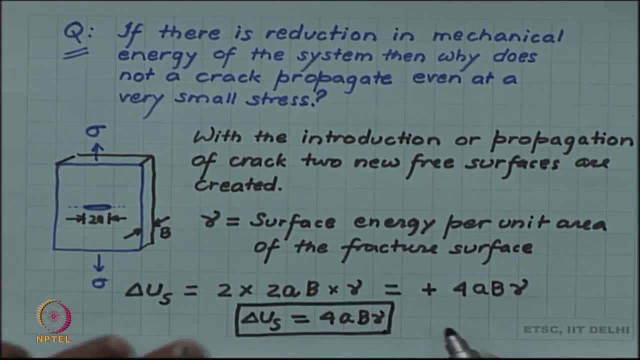 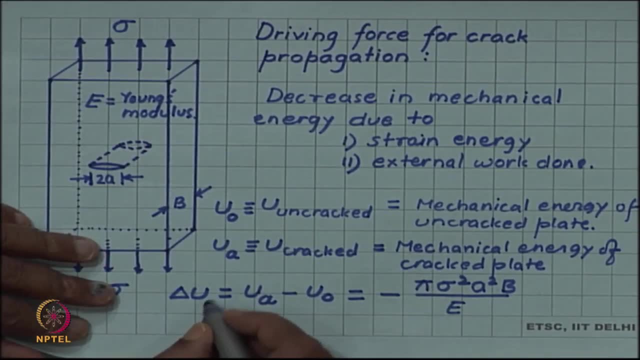 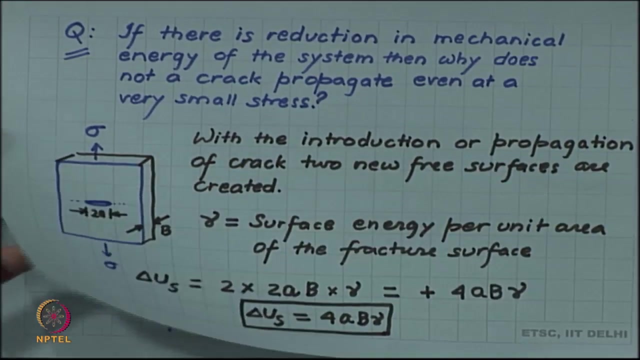 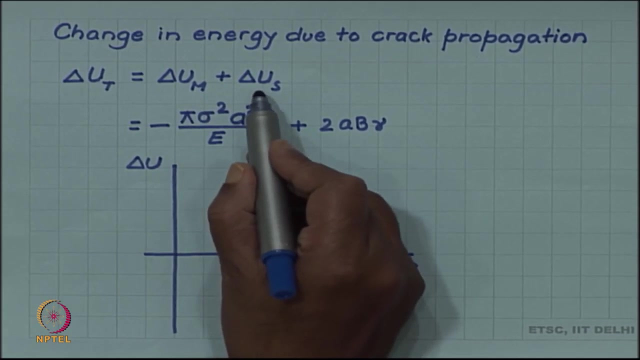 Look at the previous equation. that was a reduction in energy due to the mechanical energy, So let us call that delta u m. So now I have two component of energy change in the system: the mechanical energy change- delta u m- and the surface energy change- delta u s. We saw 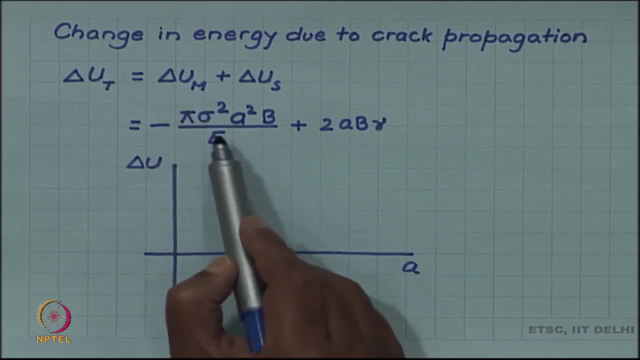 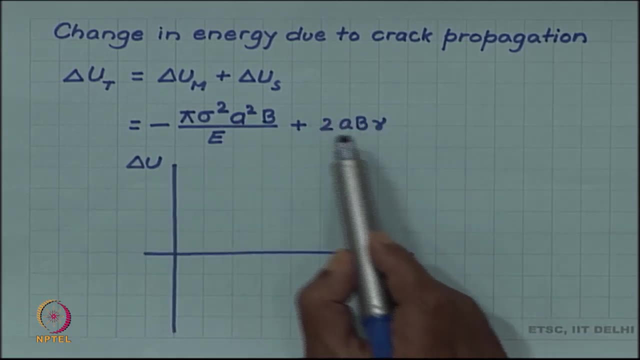 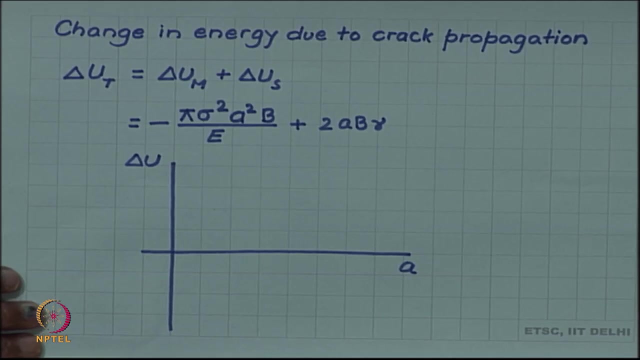 that we did not derive, but we saw that the delta u, m can be written as minus, pi, sigma, square a, square b by e, whereas the surface energy can be written as 2, a, b, gamma. Let us try to plot. let us try to plot these two energy components into as a function of the 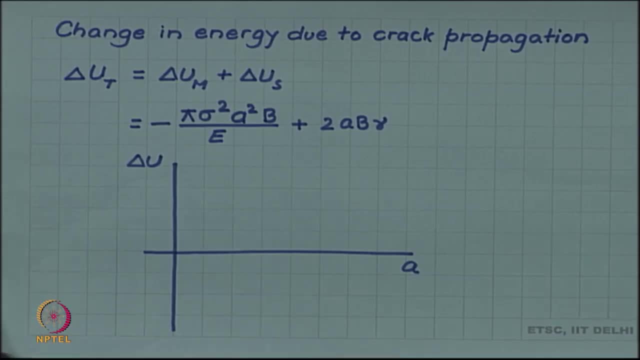 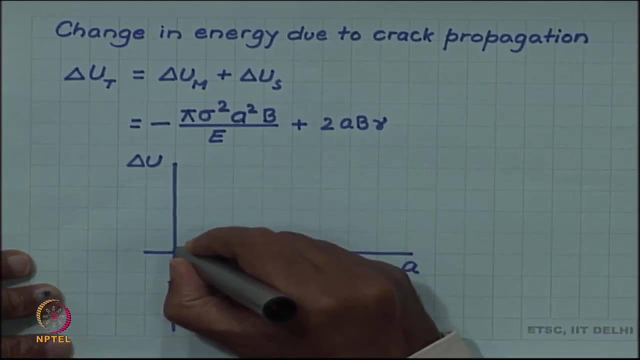 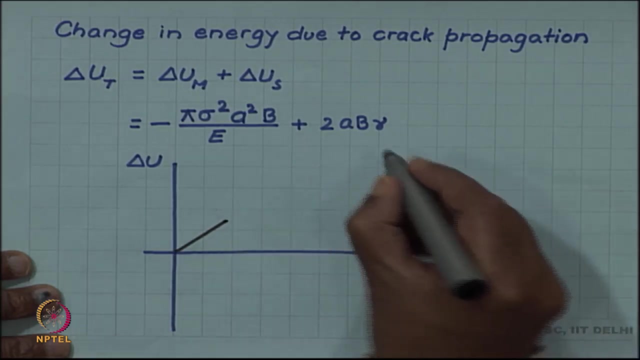 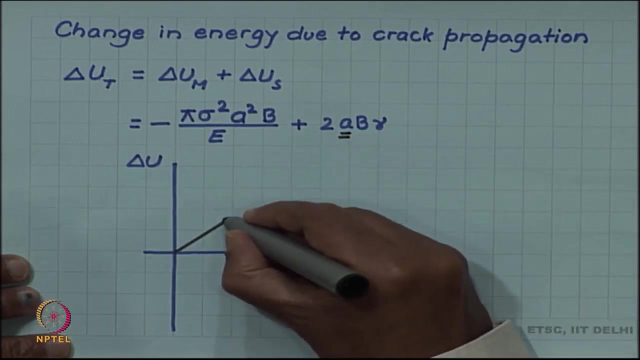 crack size. So let me first write the mechanical energy and the surface energy. Sorry, first I am plotting the surface energy. Surface energy is a easier to plot because it is just proportional to a, So it is a straight line. So I am just drawing a straight. 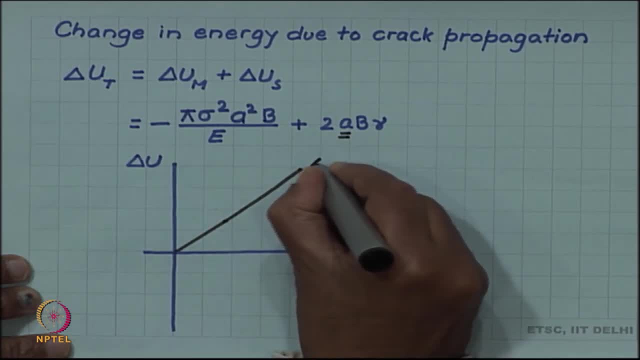 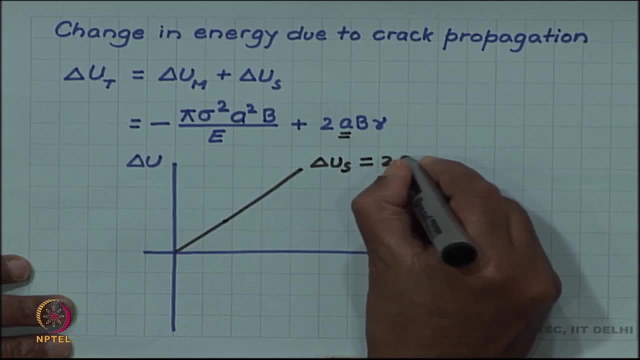 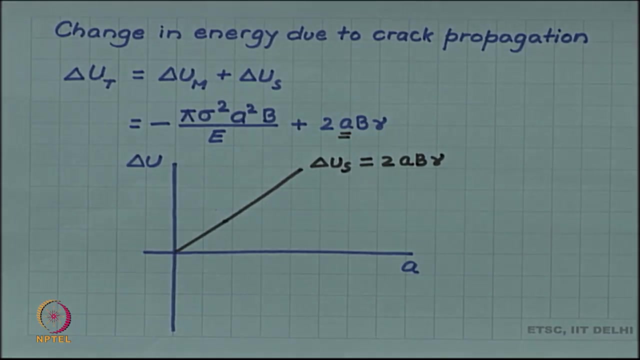 line representing delta u s equal to 2 a b gamma. So I am just drawing a straight line representing delta u s equal to 2 a b gamma. The other term, delta u m mechanical energy, is proportional to a square. So this will: 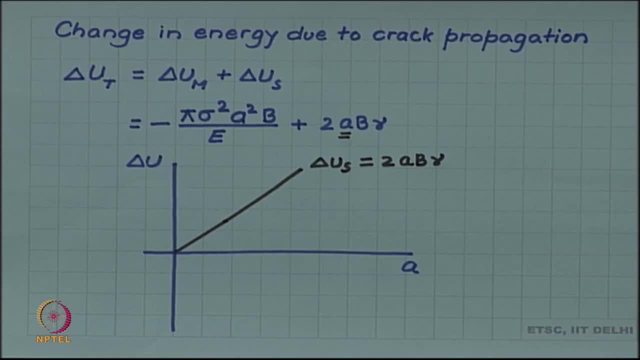 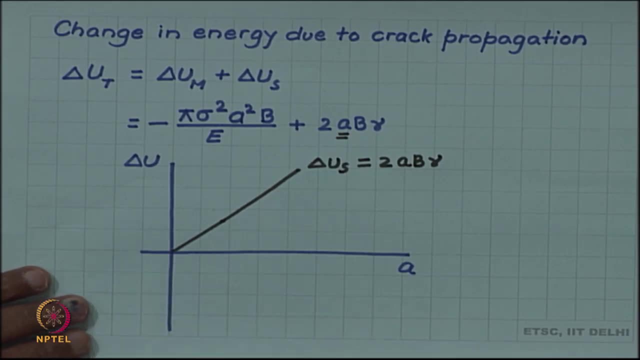 go parabolically and we can draw. it is something like this. So this is delta u m, the mechanical energy which is minus pi, sigma, square a, square b by e, The sum total delta u t will be the sum of these two and how the graph of that will look like You can see near the origin. delta u. 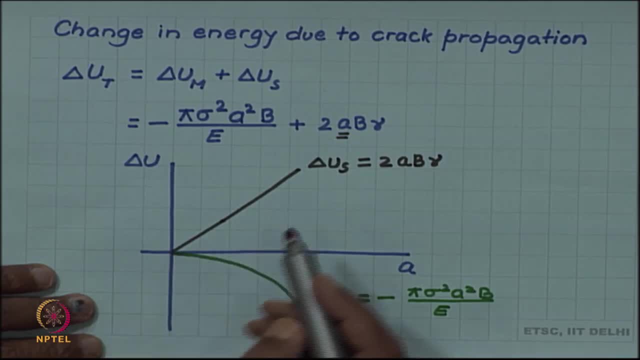 m is very small because the slope is 0, whereas delta u s is of constant slope. So initially the total will have a slope equal to that of delta u s. but gradually you can see that although delta u s is increasing with constant slope, delta u m is decreasing with increasing 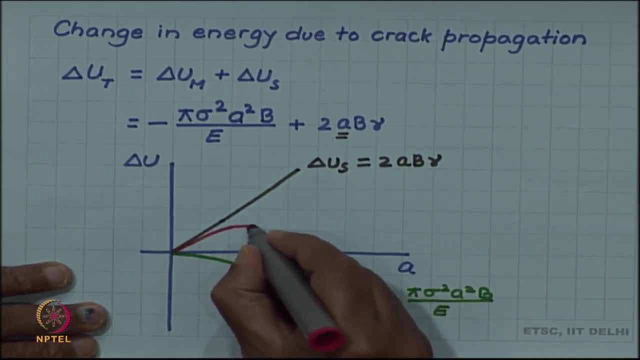 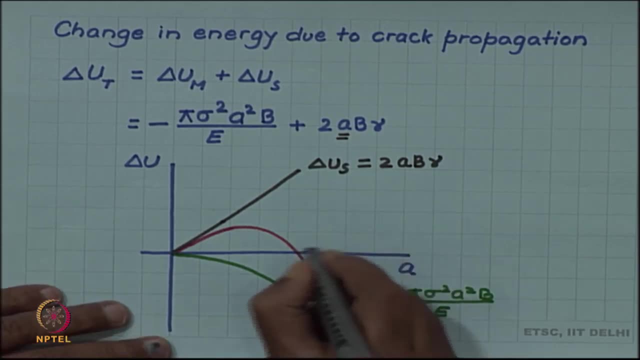 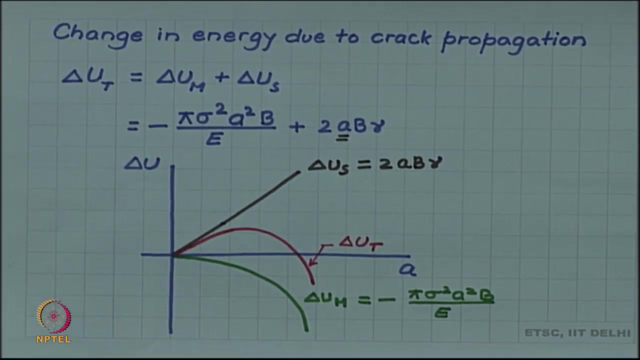 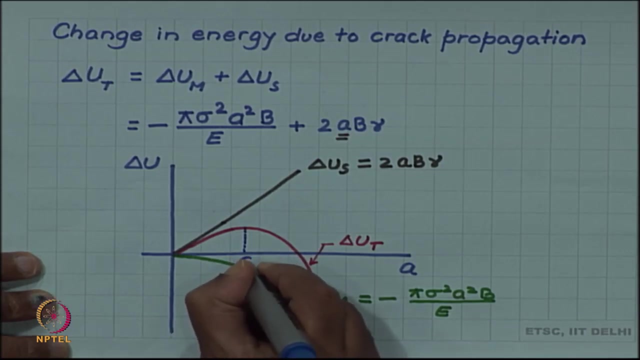 slope, So gradually it will start becoming more and more dominant and finally it will pull the curve down towards itself. So this is delta u t. you can see now that there is in this, In this curve, there is a maximum. Let me call the crack size at which this maximum 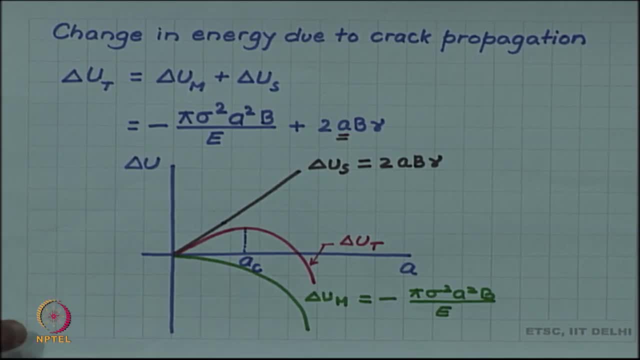 happens as a c the critical crack size. So if we now think of the situation, if you have a crack size less than a c and if you think of it growing, then the energy of the system will increase along the red curve. So a crack size is smaller than a c should not grow because 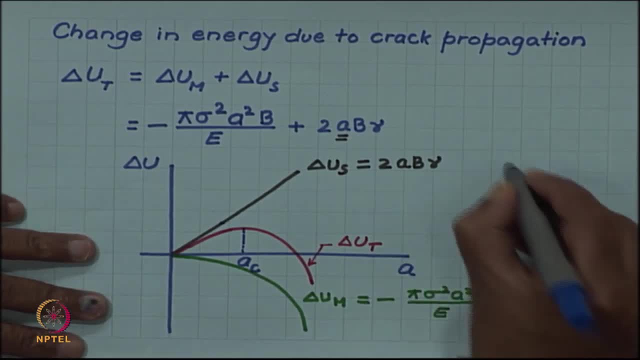 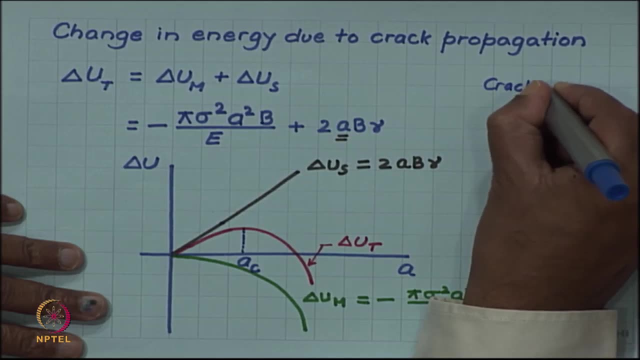 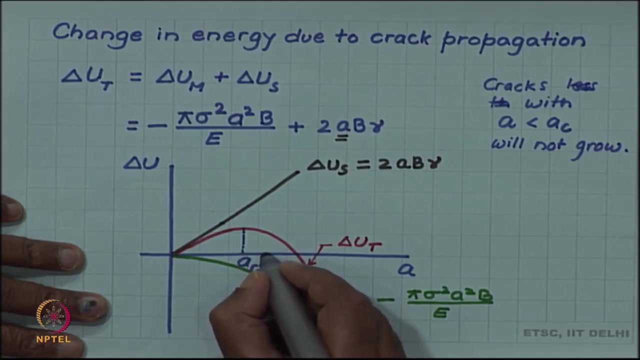 the energy of the system will increase. So cracks less than- let me write it here- cracks, or rather cracks with Cacks with Cacks, with Cacks with a less than a c will not grow, Whereas if you have a crack size larger than a c and 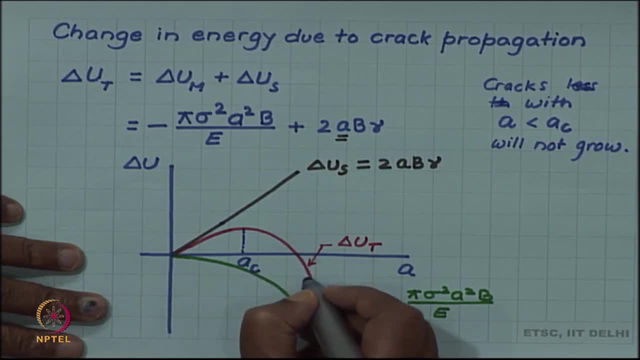 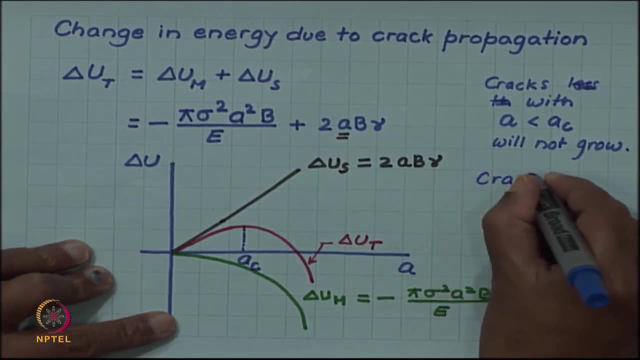 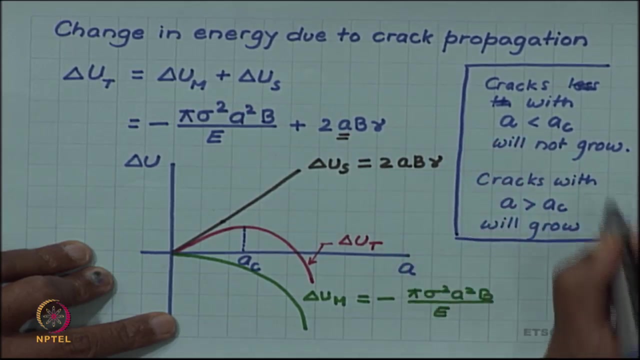 if you allow it to grow, you can see that the energy of the system will now drop along with the red curve, So cracks with a greater than a c will grow. this is a very important conclusion from this analysis. 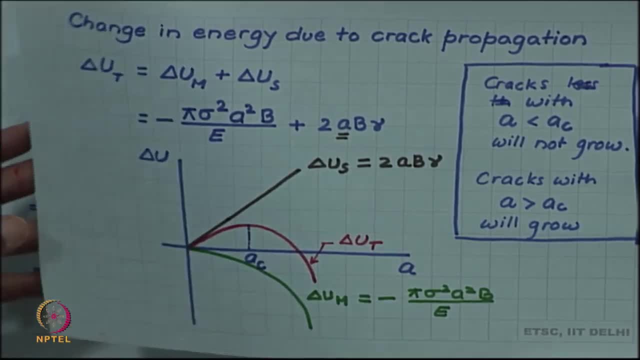 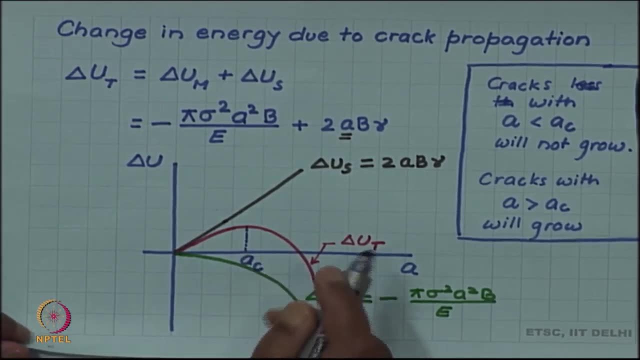 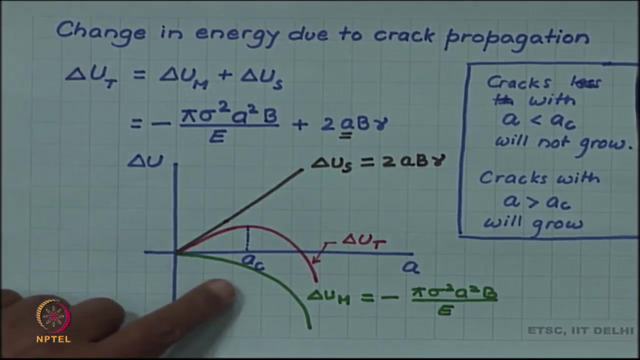 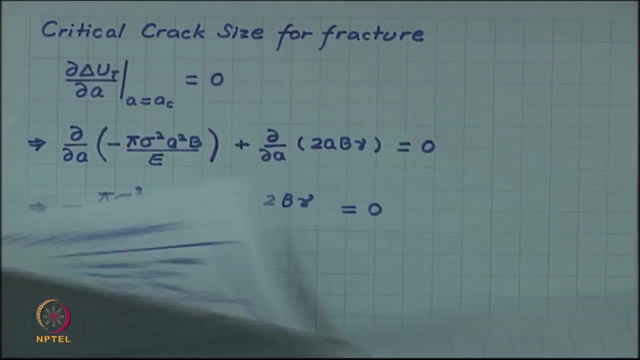 Now let us try to try to get an expression for a c Now. this is easy to do that because we already have expression for delta u t, and a c is the value of a at which delta u t is maximum. So critical crack size is where a c is greater than a c and delta u t is greater. 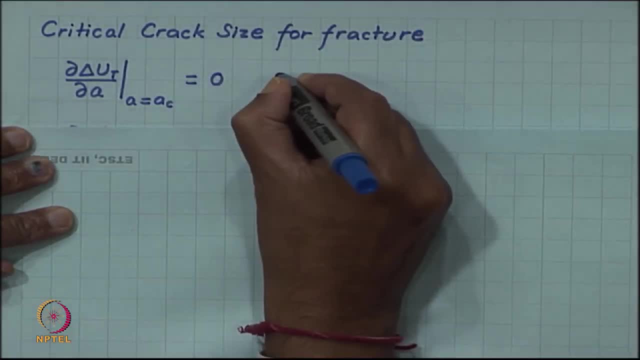 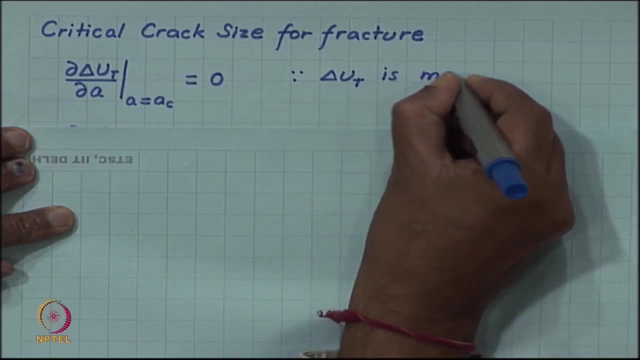 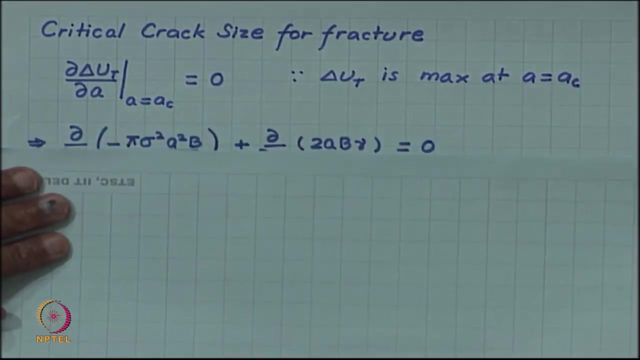 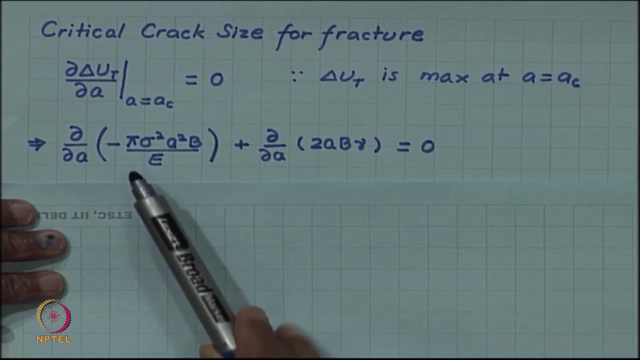 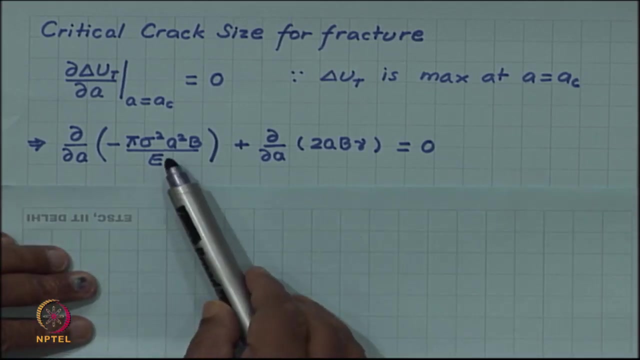 than a, c. So we can easily do this differentiation. they are 2 simple terms, the mechanical energy term and the surface energy term, And both of them are completers, same eras. both of them are simple function. one is a square, another is a. So we just differentiate. 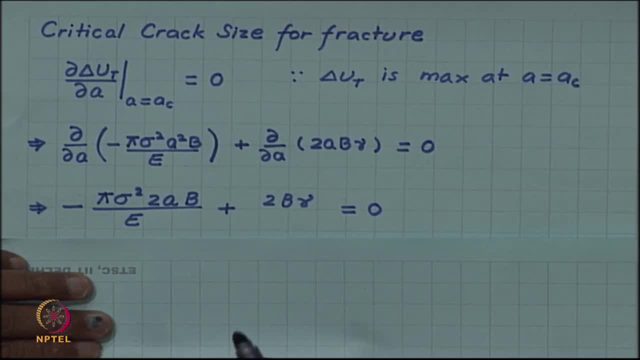 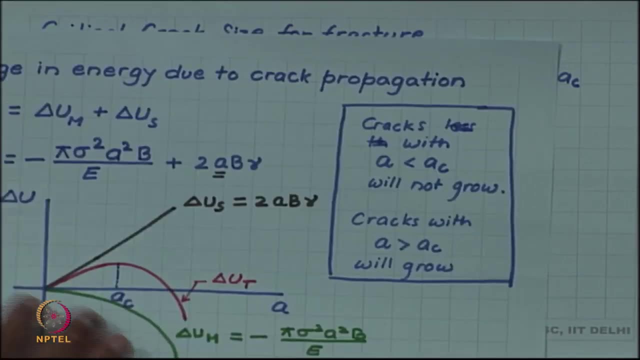 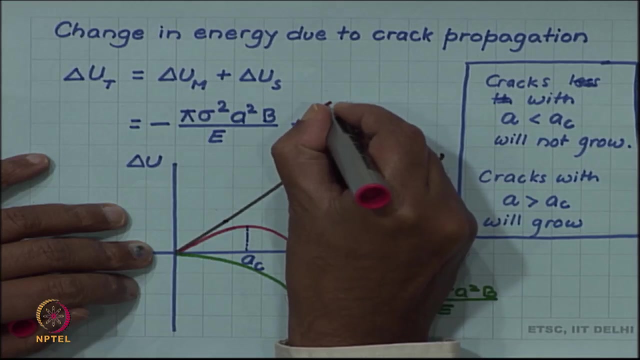 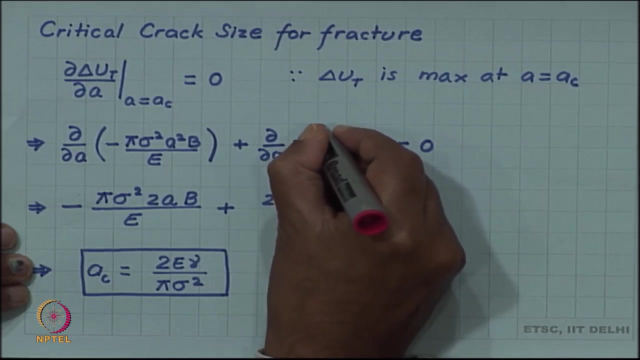 a square differentiates as 2 a. I just made a mistake here. here also I had made a mistake, So let me correct that this is not 2 a b gamma. this is 4 a b gamma. this is also 4 a. 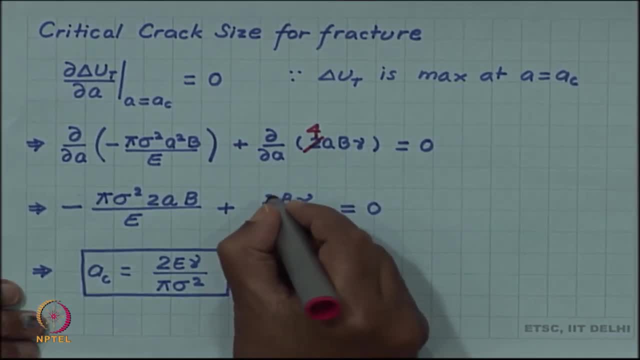 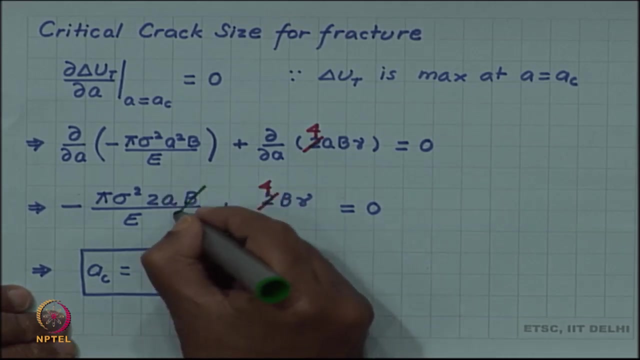 b gamma. So after differentiation we get this. and if we now solve it for, So you can see, b will cancel with b and 2 will cancel with this 2.. So you will have a c as 2 e gamma by pi sigma square. So you have an expression for the critical. 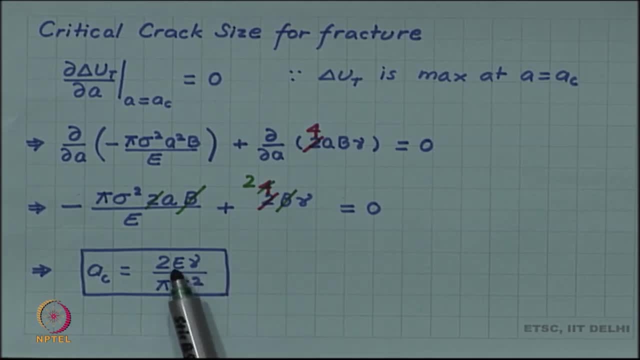 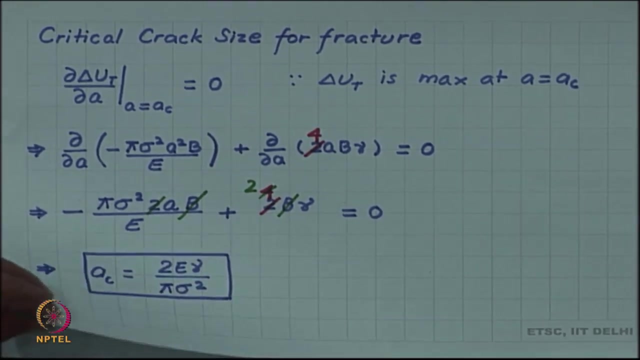 crack size in terms of the properties of the material, the elastic property, the modulus and the surface energy, as well as the mechanical stress, which you have applied sigma. So we have got an expression for critical crack size and let us see what are the consequences of this expression. 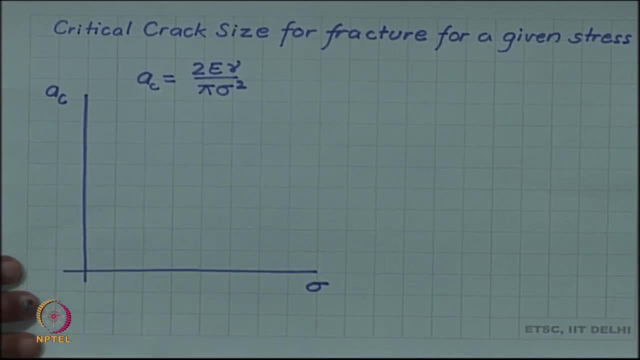 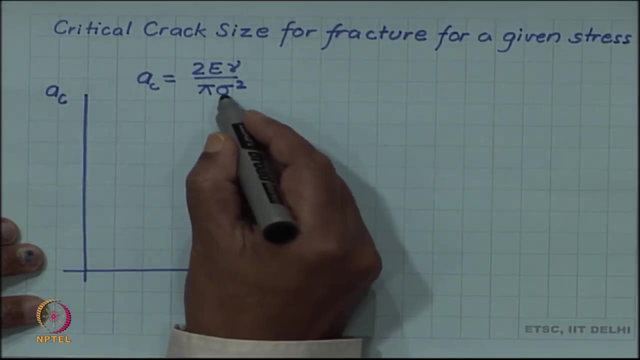 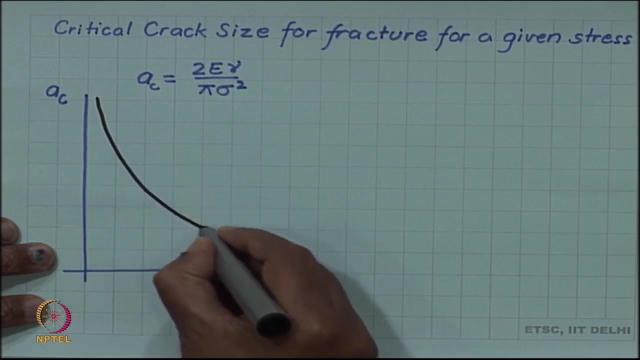 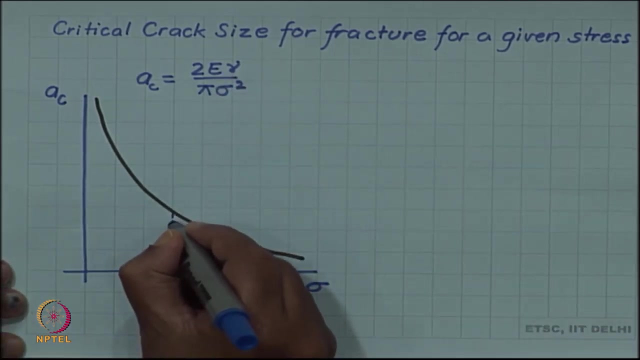 So if we plot this curve, if we plot this curve a, c, as a function of sigma, you can see, with increasing sigma, So sigma will keep decreasing. So you have, you have a curve like this. how do we interpret this curve? let us see, this is telling us that for a given stress. So let us, let us assume. 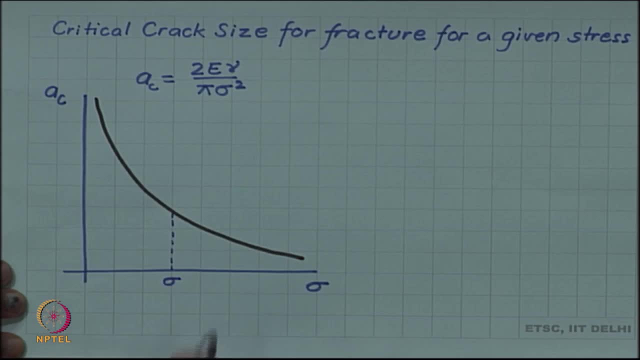 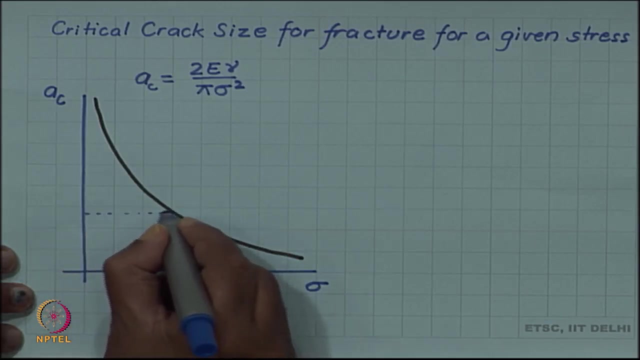 that we have this stress sigma applied, Suppose we are applying this stress, and then this is for that applied stress. this is the critical size. this is the critical size. So if the actual crack size is- let us say this- if the actual crack size is this, then we can see that for this. 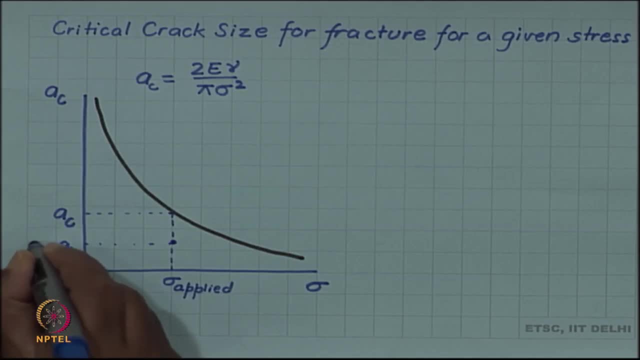 This is the actual crack size, a. So a is less than a c and we have already seen that for such cracks, such cracks will not propagate, for this applied stress. So this will be the case everywhere below the curve. if you have a point below this curve, the crack of 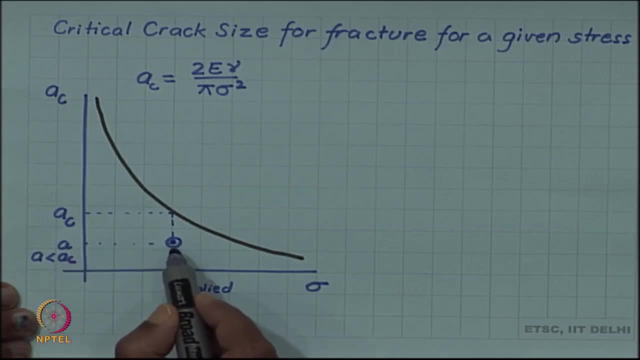 that length will not be growing or increasing in size for the corresponding applied stress. So this region below below this curve is a safe region. So let me write this with green: this is safe region. However, for the same applied stressful. 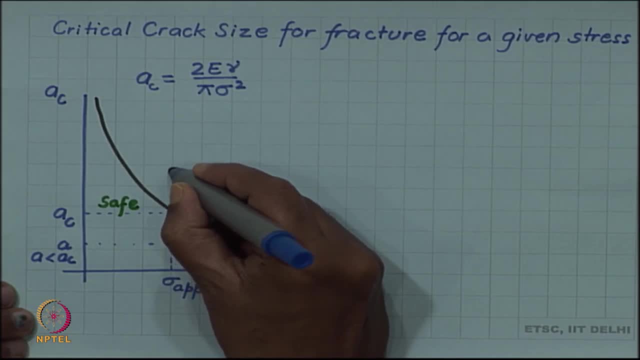 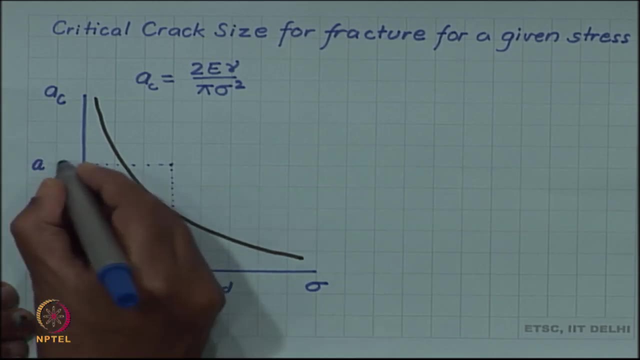 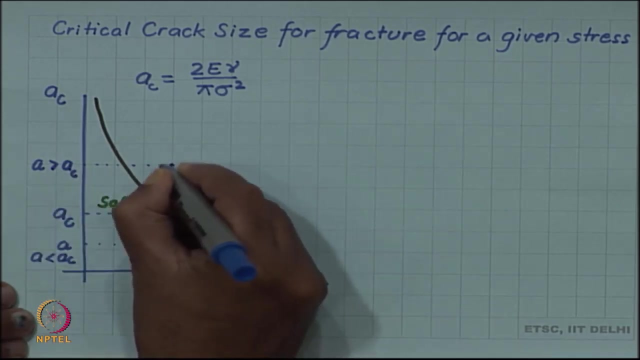 if we have a crack size which is higher, if we have this crack size which is greater than AC, Then obviously this crack, according to our analysis, or according to Griffith's analysis, this crack will propagate and will cause fracture. So this: 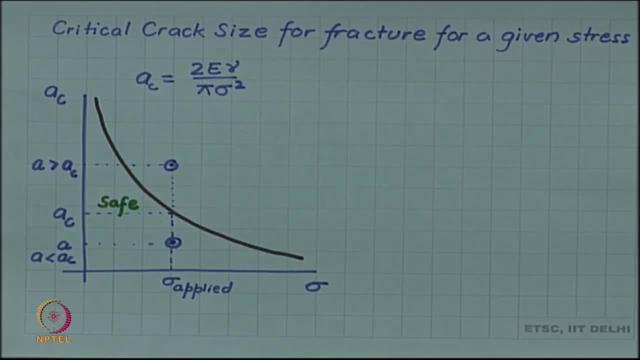 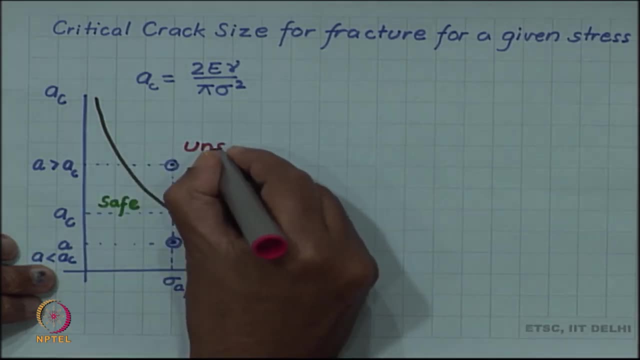 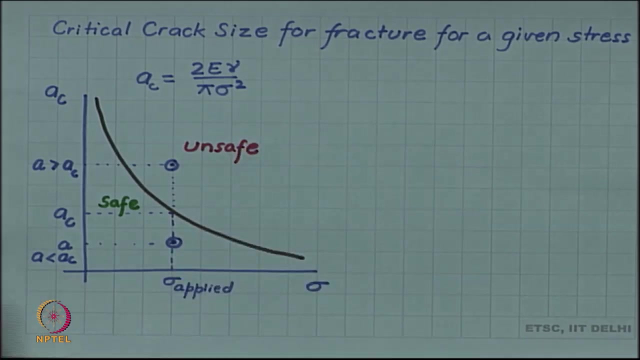 region is unsafe. let me mark it with red and this will be true for everywhere above this black line. so this is an unsafe region. So in the AC sigma domain, this line- AC versus sigma line- divides the AC sigma space into two domains: the unsafe domain and the safe. 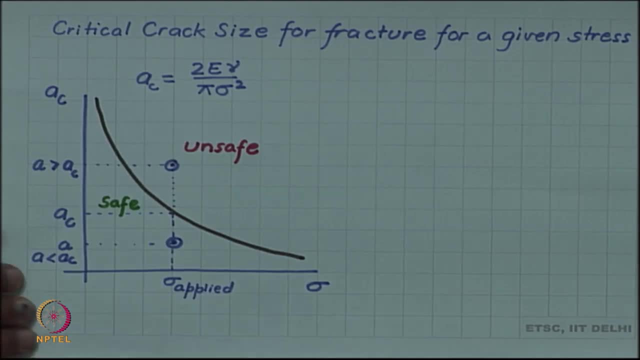 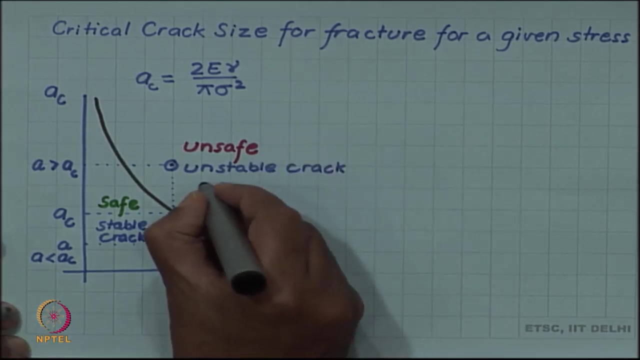 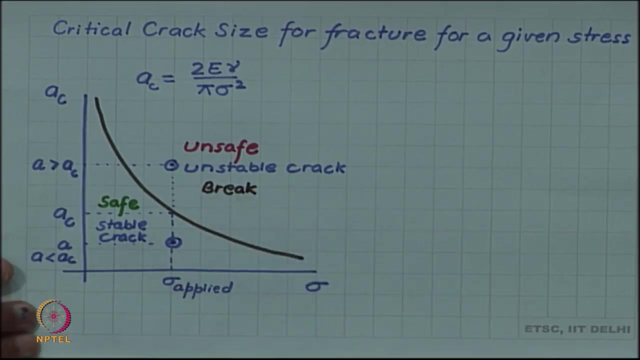 domain. We can also write this as unstable crack, because this crack will propagate, and whereas this we can write as stable crack, this crack will not propagate. Thus, here the component will break, where here, although the crack may be present, but the component 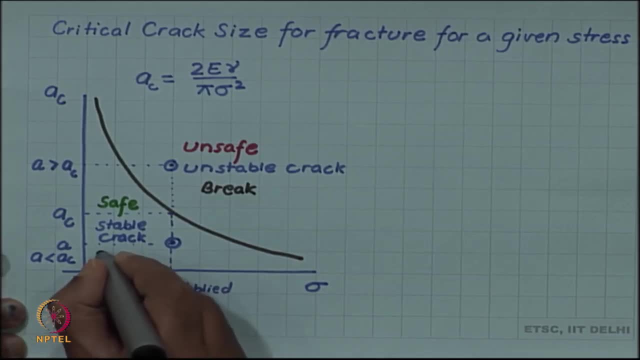 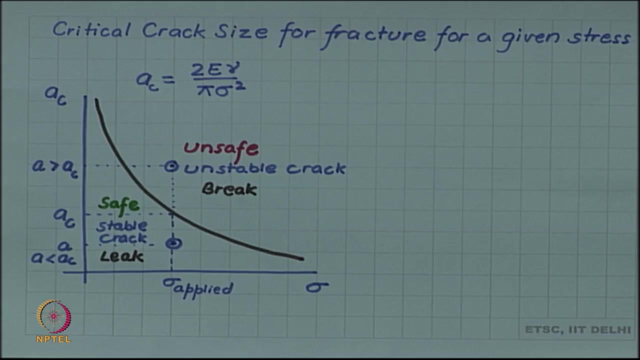 may not break. and if it is a component, like a pressure vessel, then it will have leak. So it will leak but it will not break. and here above the curve it will break. So this is an important information coming from the Griffith's analysis of the crack problem And you can see that the stress here in from 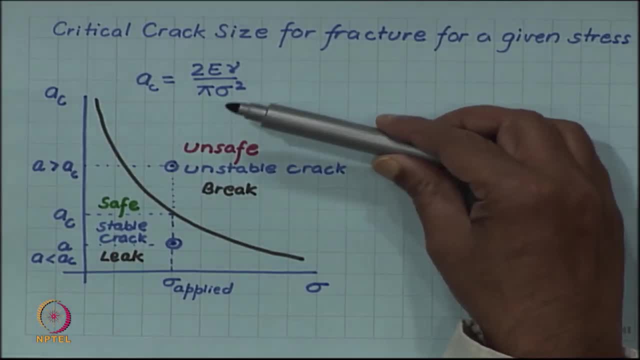 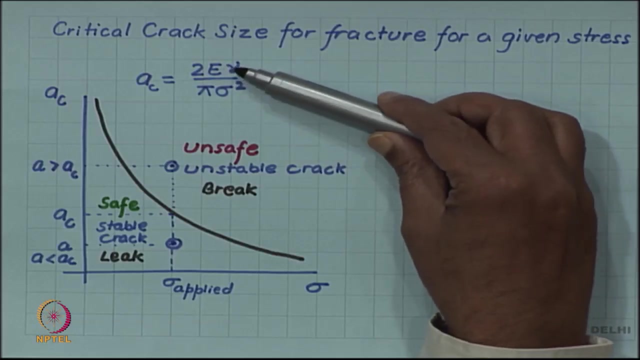 this expression you can see: stress was the driving force for crack propagation. So larger is the stress, smaller is the critical size. So if you have larger driving force, even smaller cracks can propagate. but the surface energy was in a sense a barrier or 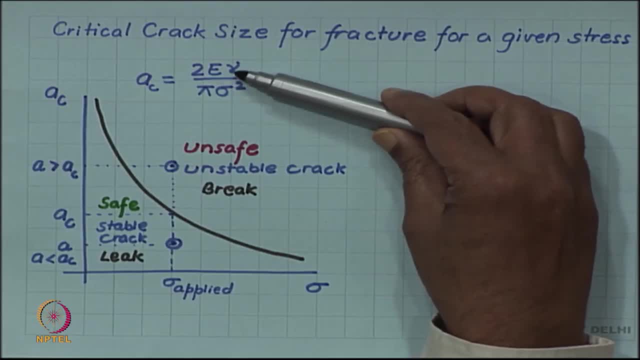 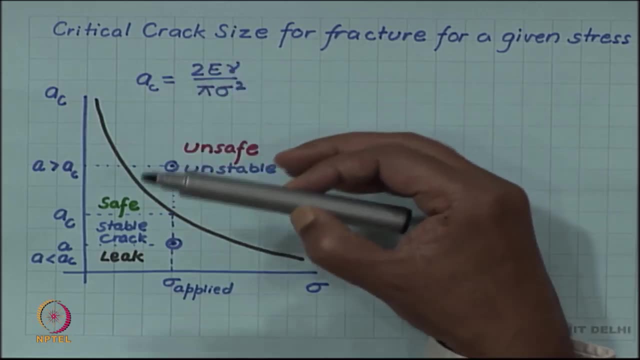 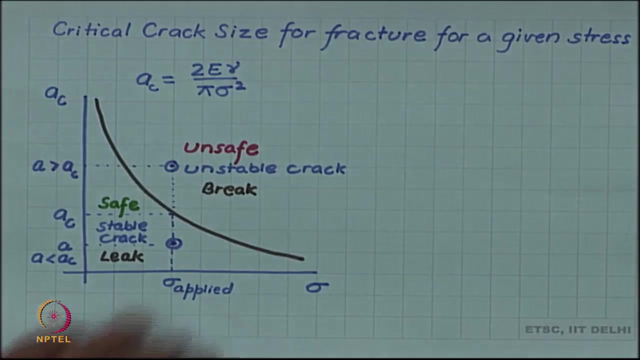 opposite. So this is an obstacle to crack propagation. So larger is the surface energy, higher is the critical crack size. So if surface energy is larger, only the small cracks will not be able to propagate. only correspondingly larger cracks will be able to propagate. We can look. 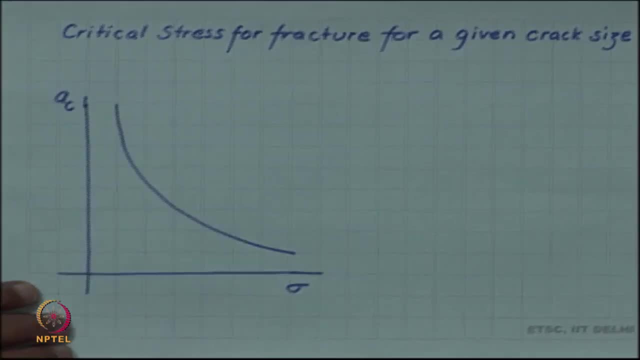 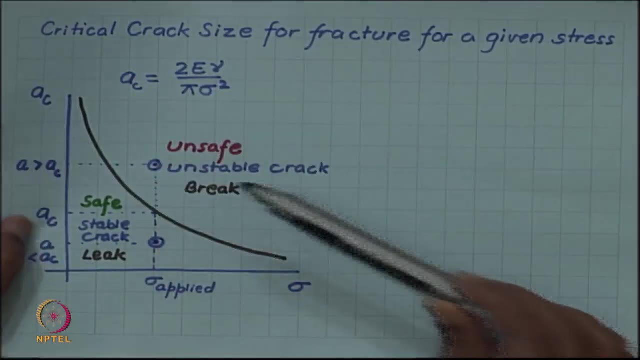 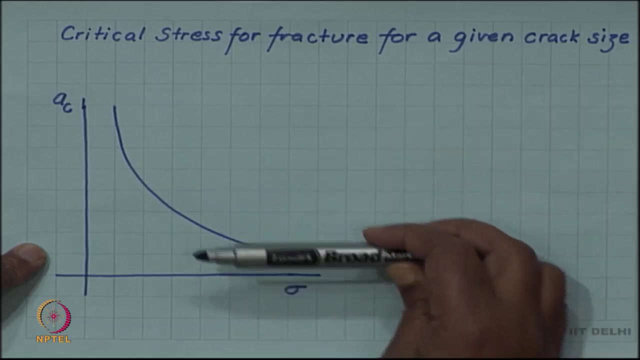 at this curve in a slightly different light. Instead of looking at it as critical crack size as a function, As a function of given stress, which is what we have drawn here, we can change our point of view and try to look at stress as a function of crack size, critical stress as a function. 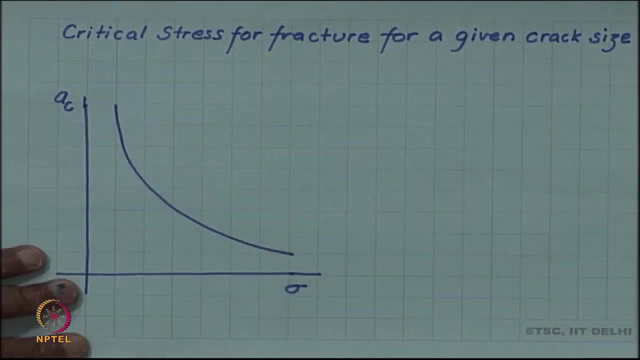 of crack size. And this interpretation is possible because, again, if you look, we said that for a given stress, for a given stress, this was the critical crack size. So this was the critical crack size. Now suppose I change my point of view and I simply call: 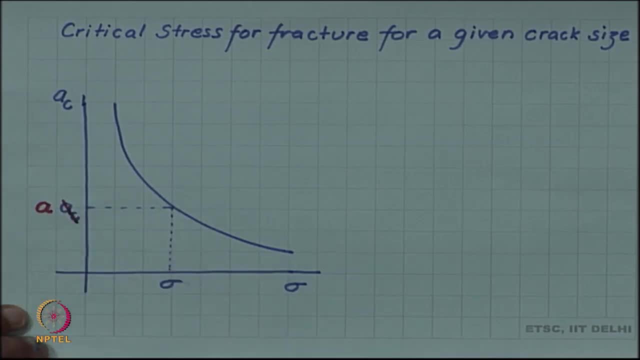 not this as a critical crack size. I do not look at it as a critical crack size and I say that I have a component in which this is the crack size And I want to know- and I am gradually applying higher and higher stress- at what stress it will fracture. So 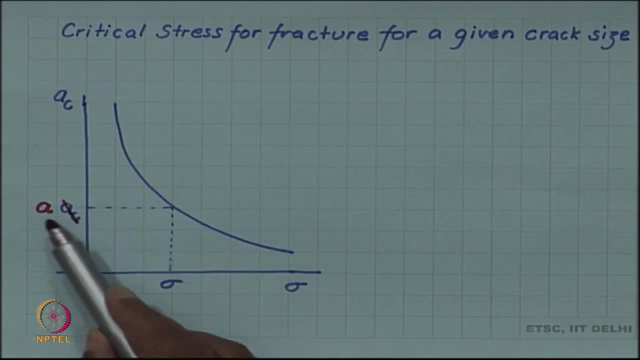 what is the critical stress for fracture, for a component? So this is the critical crack size, the component with this crack size. Now, we have already seen that at this stress, this was the critical crack size. Now, if I start with this stress, if I start for a 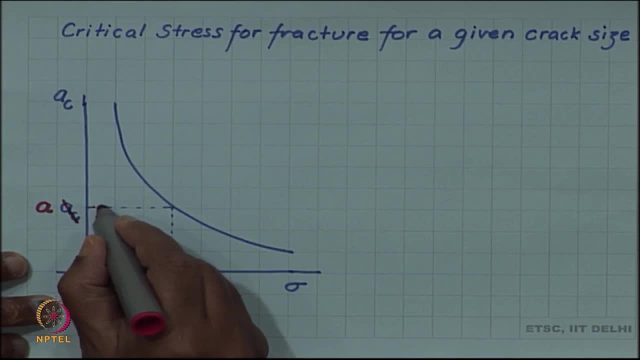 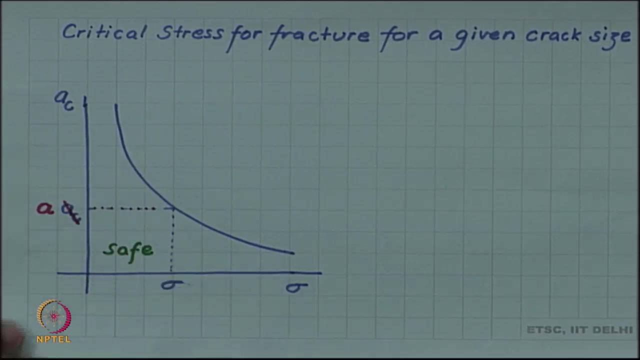 given crack size- and I start with zero stress and gradually increase this stress, you can see that I will remain in the safe region. We had seen that this was the safe region below the curve, So I remain in the safe region till I hit the curve again. beyond that, 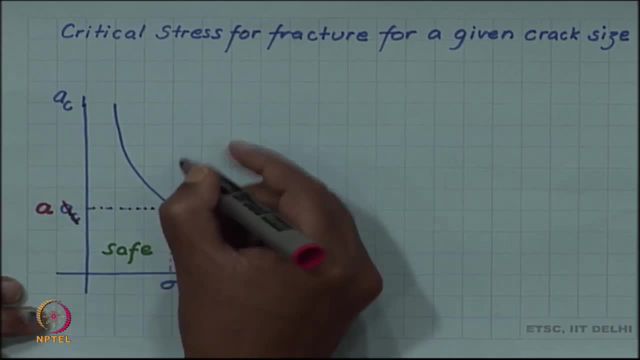 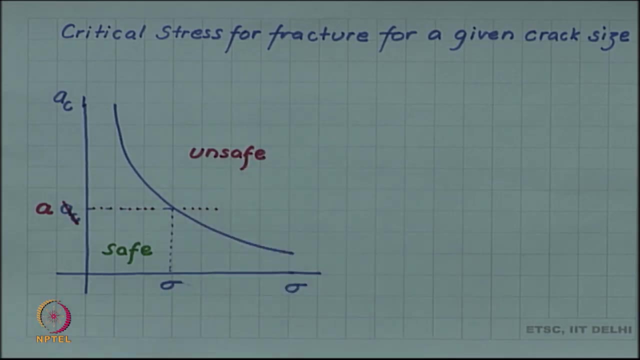 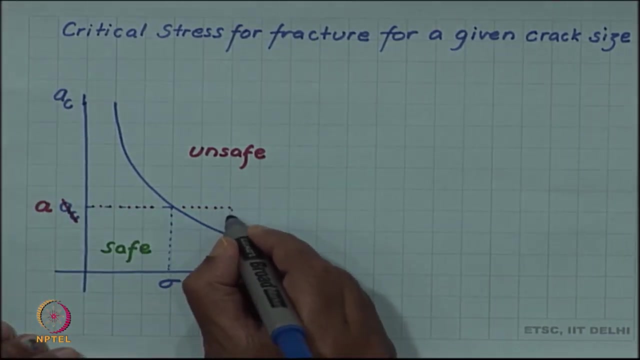 if I go beyond that, if I go, I will enter the unsafe region or the crack propagation region. Because for those stresses you can look at it another way, that if I have an applied stress, this, then the critical crack size was much smaller. a c was much smaller, and then this: 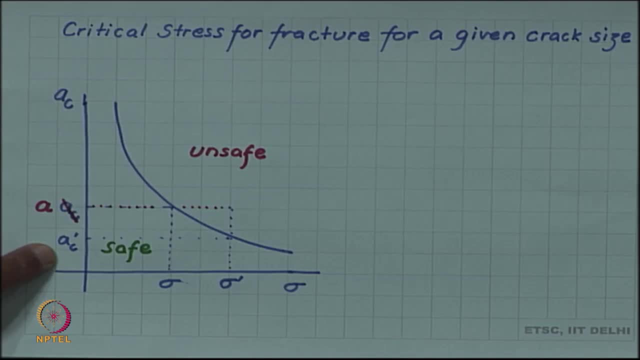 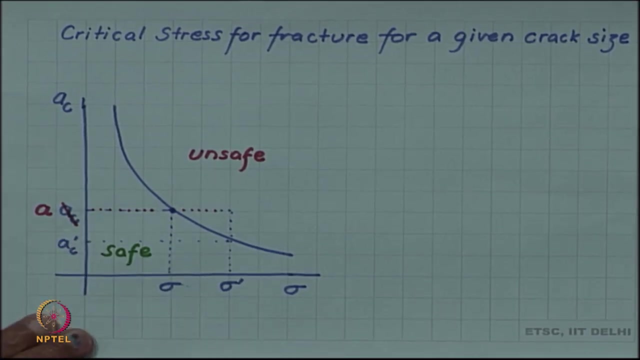 a is larger than a. c for this applied stress. So you will be in the unsafe region. So the stress dividing the safe and unsafe region is again given by the same curve which we have plotted as A, c versus sigma. So now for this: given a, this becomes sigma critical, which we label. 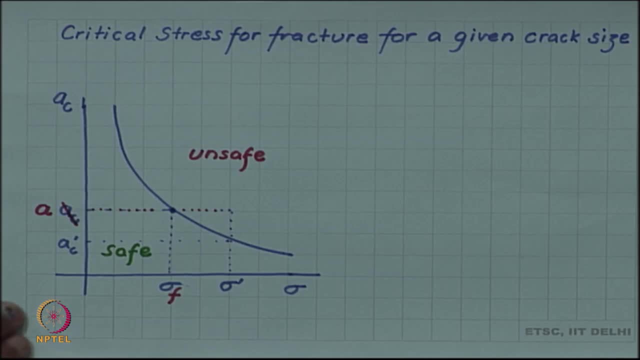 as sigma f. So now I change the interpretation of this curve. instead of calling this an, a, c versus sigma, I call this as a versus sigma f. So for a given crack size, I can find what is the critical crack stress, And it is the same equation, same curve, So I can write an expression for sigma f simply. 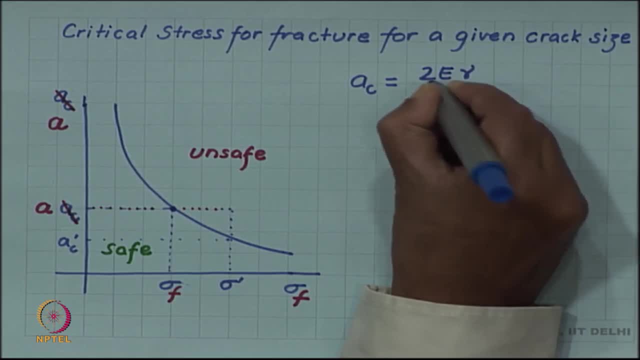 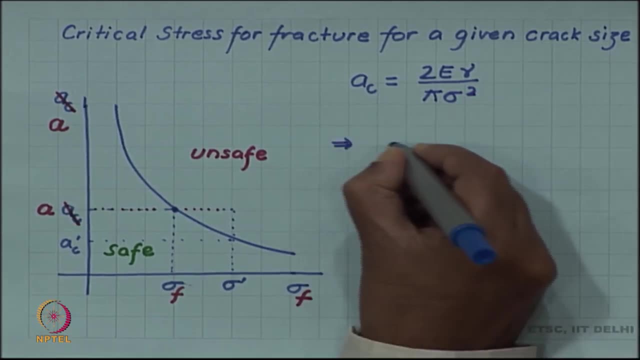 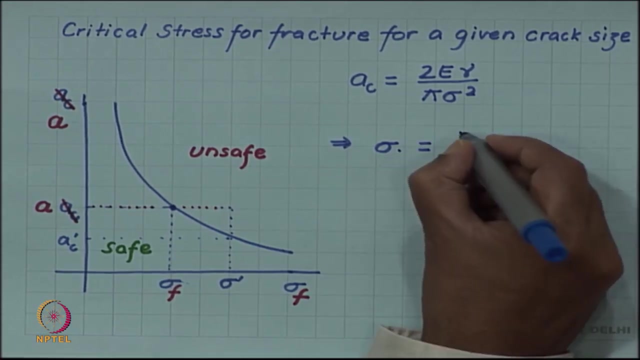 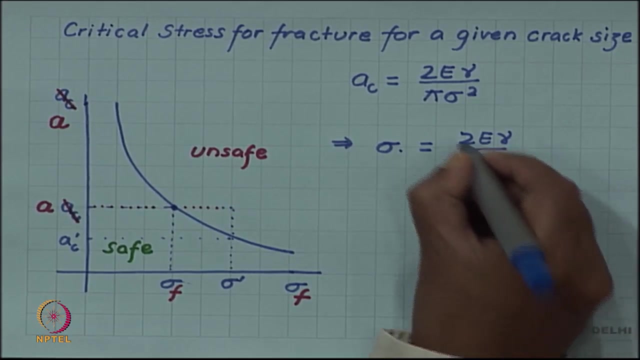 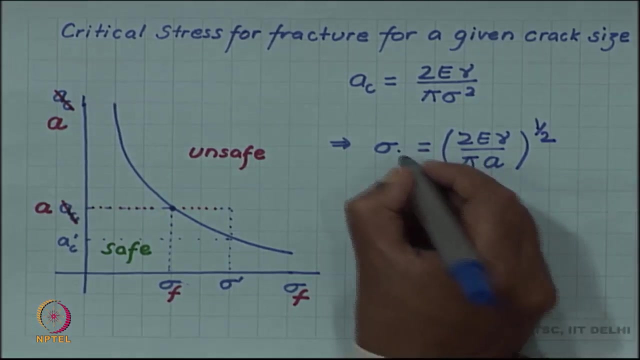 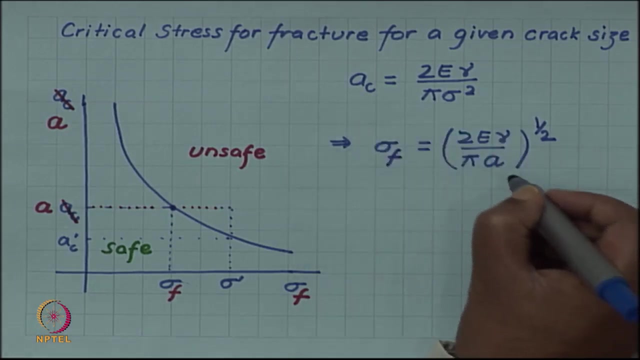 by algebraic manipulation of this equation. all I have to do is now solve this for sigma. So I get 2 e gamma by pi, a square root, and I write now, since I am, my interpretation has changed. So sigma has now become the critical stress, sigma f and a c has become the given crack. 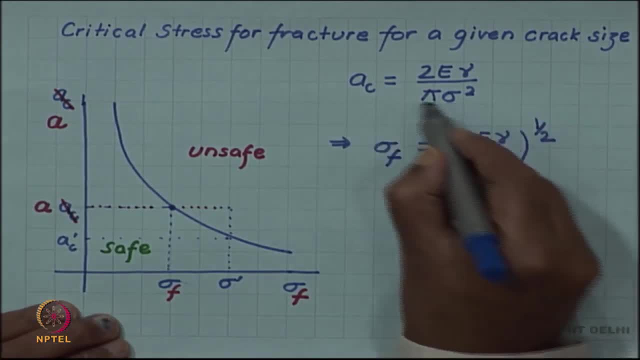 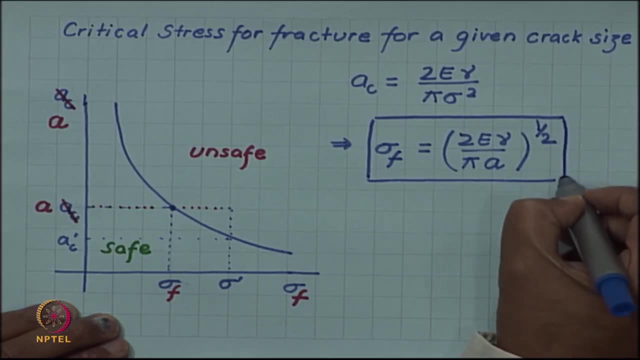 length a. So this expression also is known as the critical stress sigma f. So this expression also is known as the critical stress sigma f. So this expression also is known as the Griffith's equation. So both are Griffith's equation, either in terms of the critical crack size or in terms 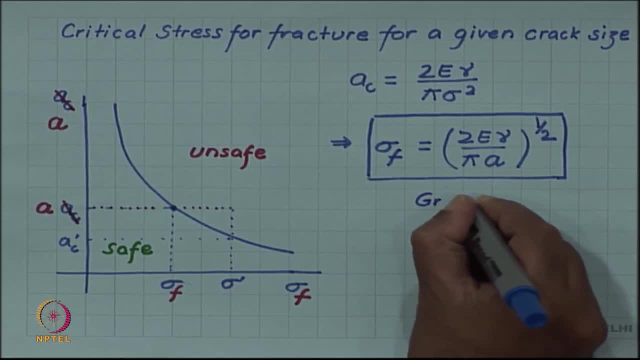 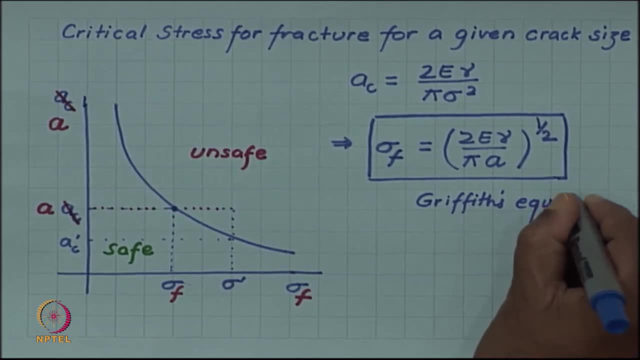 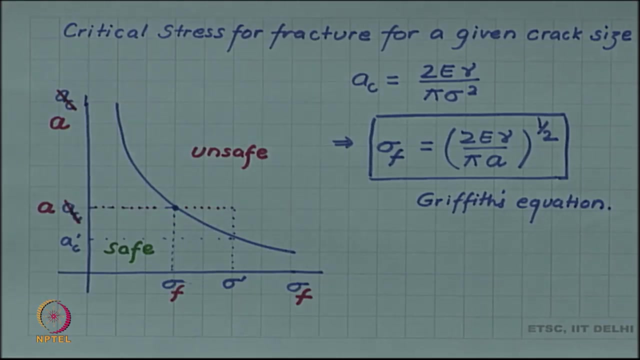 of the fracture stress. So to summarize, it was Griffith's central contribution to realize the importance of surface energy as an important factor in the analysis of crack. So the mechanical energy is the driving force for the crack, reduction in mechanical energy, whereas increase in surface energy is obstacle to the crack propagation.